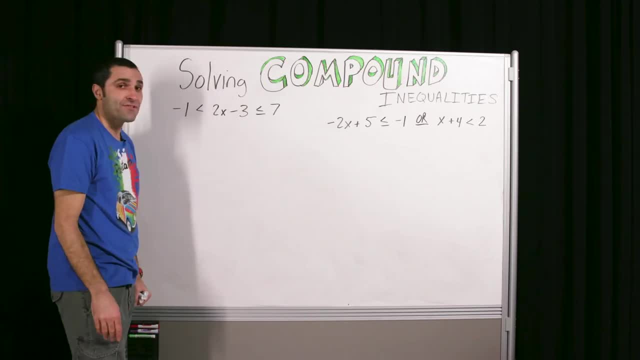 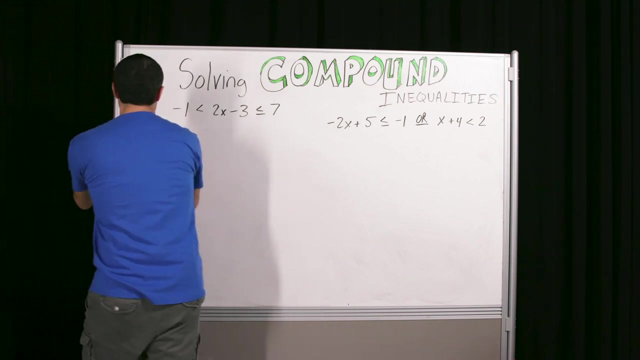 This one needs to be true. So the answer is: and Okay. So if you look at it closely, we could have said we could break this into two, And a lot of people actually like to see it this way. My eraser, here we go. They like to see negative one less than 2x minus. 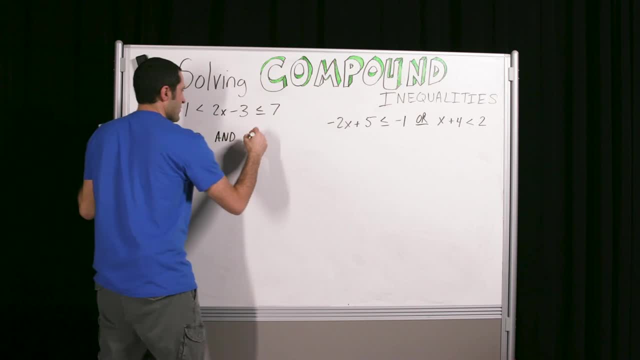 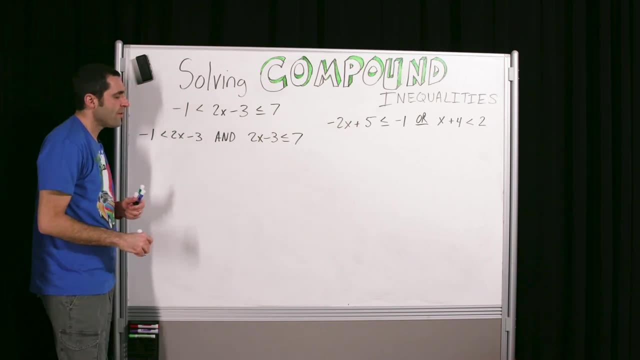 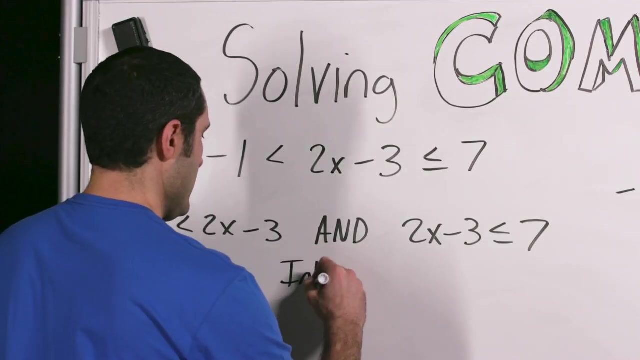 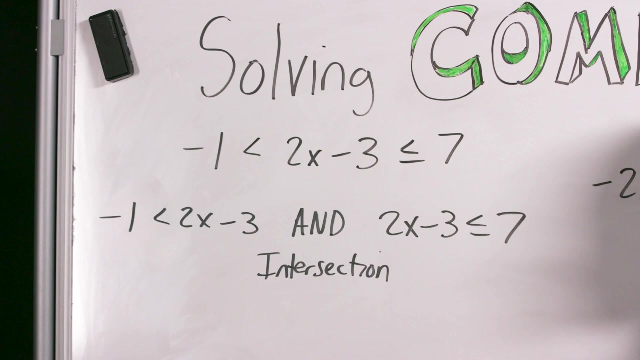 three and 2x minus three less than or equal to seven, And that's totally fine. You can solve both, Okay. This word- and, by the way, is code for intersection, Intersection, Intersection, Right, And by intersection it means both need to be true at the same time. Okay, There's. 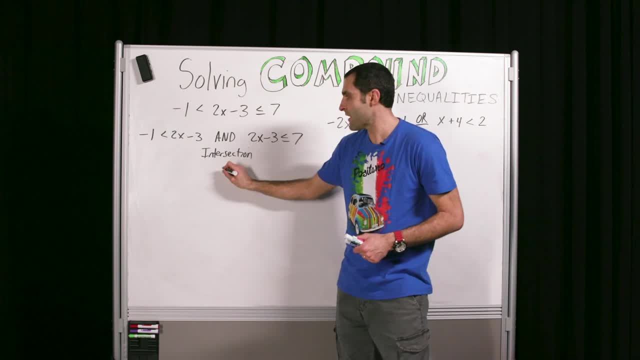 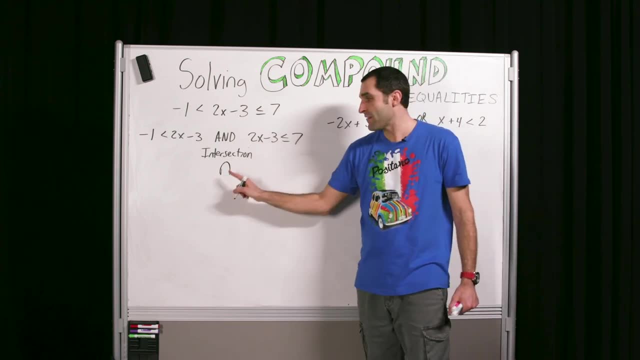 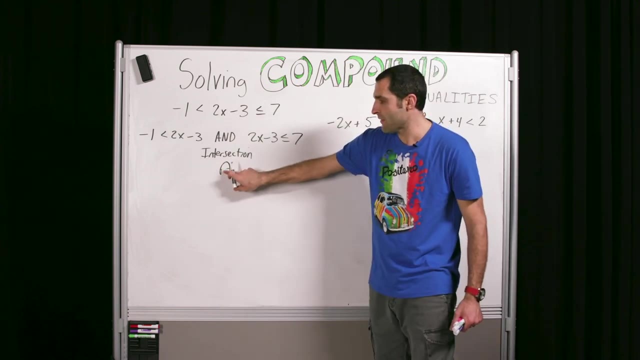 a fancy symbol for intersection. Basically, it looks like this: All right, That's the symbol for intersect, And the reason that I can remember this is that I just think of it like loop. It looks like an ant, you know So, but you don't put that there. It's just. 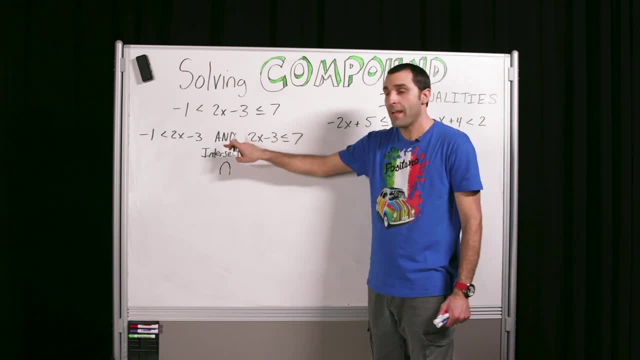 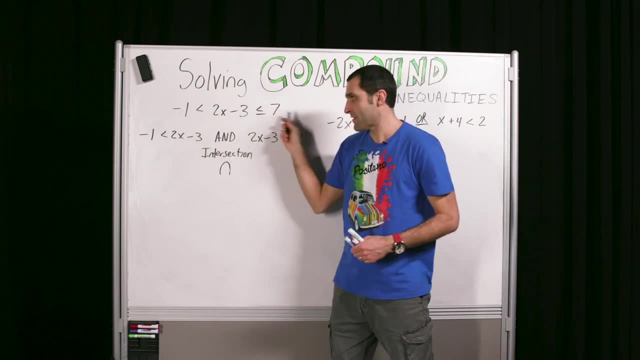 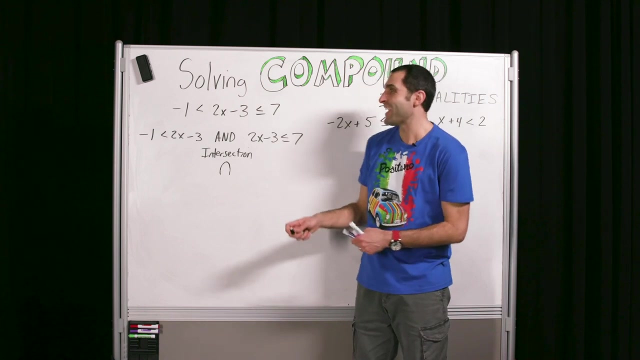 for us to know. So this thing means intersect, which is code for ant. Both need to be true. However, what's cool is that you can solve this little sandwich. I like to call it the s-andwich: Get it, Get it. 2x minus three is sandwiched between the negative one and 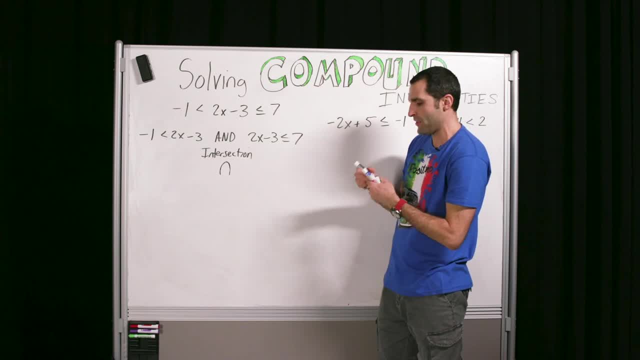 the seven. Okay, So this little sandwich can be solved algebraically. Let's put it down, It's fun Sandwich. Okay, So this little sandwich can be solved algebraically. Let's put it down, It's fun Sandwich. 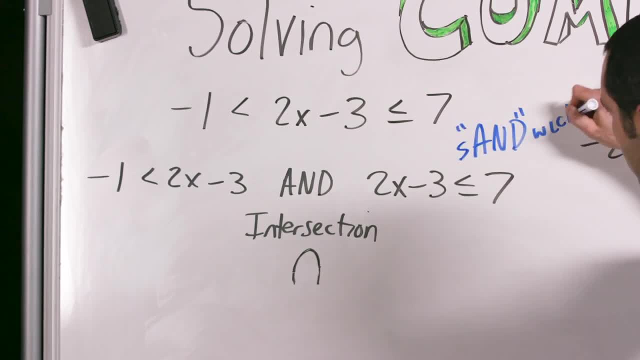 and which, meaning that if you see this sandwich thing, you know that it's an, and okay, teach your tricks. so let's isolate x, all right. in order to do that, we need to get rid of the two and the negative three. we've learned in previous videos, algebraically speaking, that we want to move this. 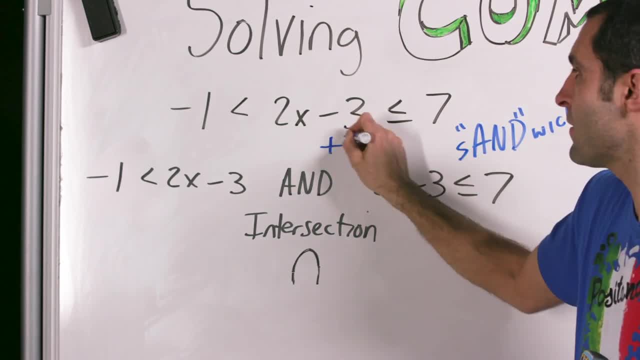 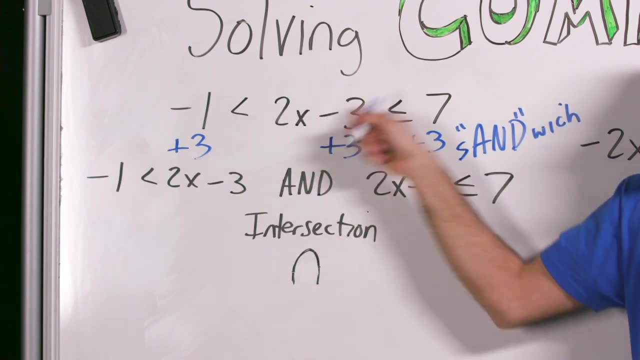 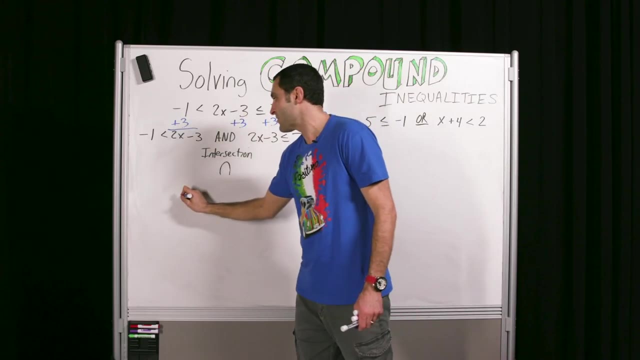 three over first by adding three here and here and here. you could add three to all three components and it'll level out. it'll be even all right. i'm going to bring the work down here. negative one plus three is two less than comes down. this is just like a little aside, so let me put that in. 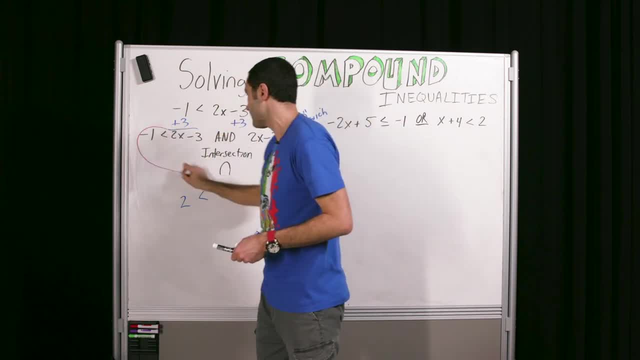 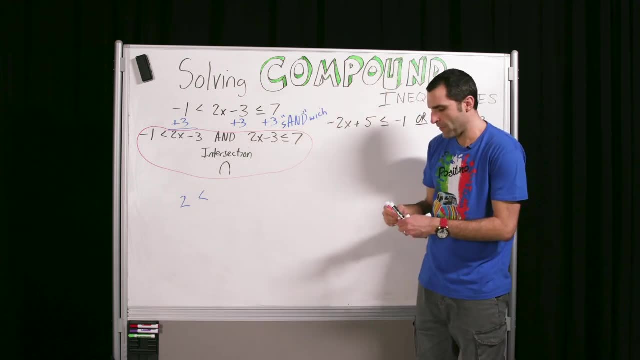 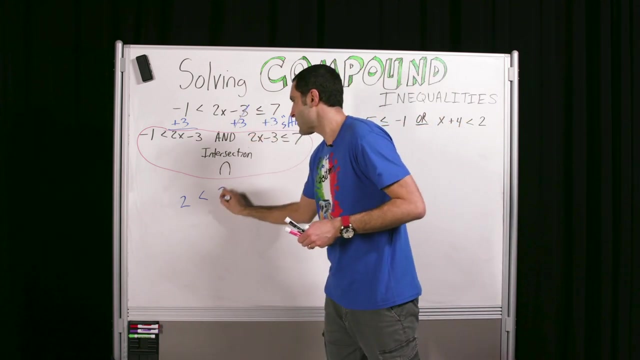 like a pink box. just so you see, it's another way of looking at it. so there you go. so that's equivalent to this, but now that we're coming back in negative two, we can switch to blue. these go is less than, 2x less than, or equal to 10, and we are one step away. 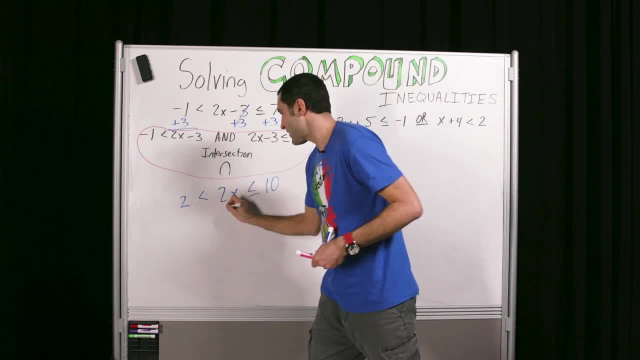 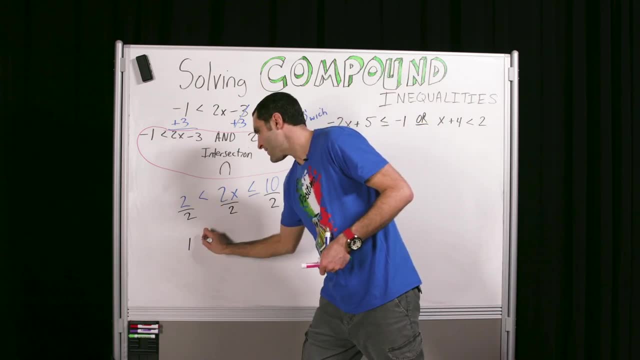 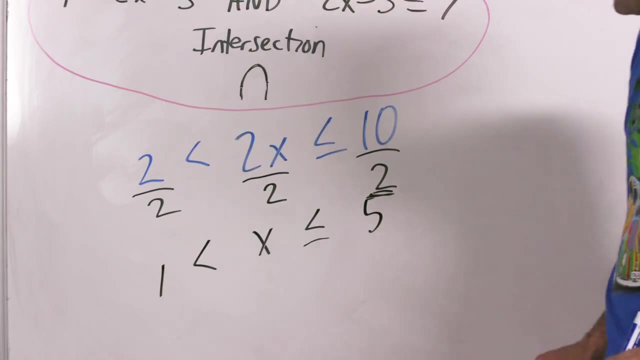 we're going to divide everything by two, so this goes two and here and here divided. so two divided by two is one less than x less than or equal to 10 over two five. so what this is basically saying is that x is sandwiched between one and five, and 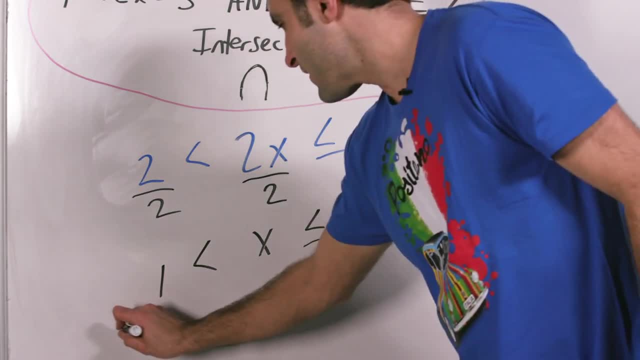 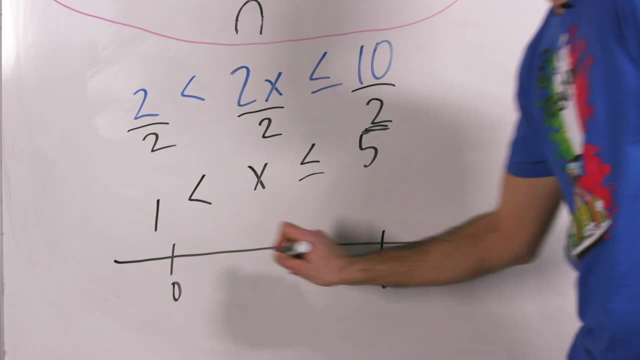 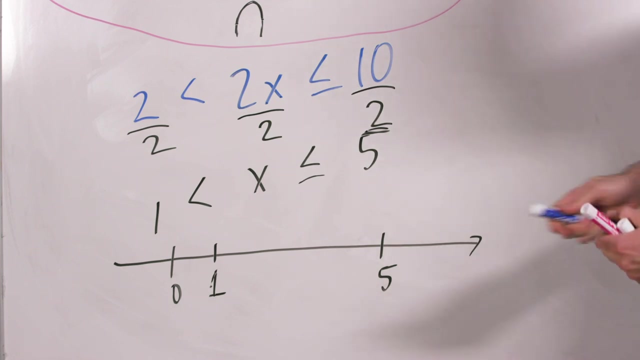 your next goal will be to graph this on a number line. it's pretty cool. so if we have zero here, you have like five here, we have one here. x is essentially between the two, not including one. so when we want to not include a number line, we're going to have to add a number line to the 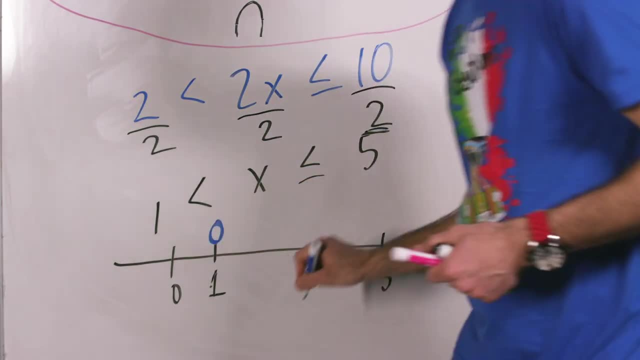 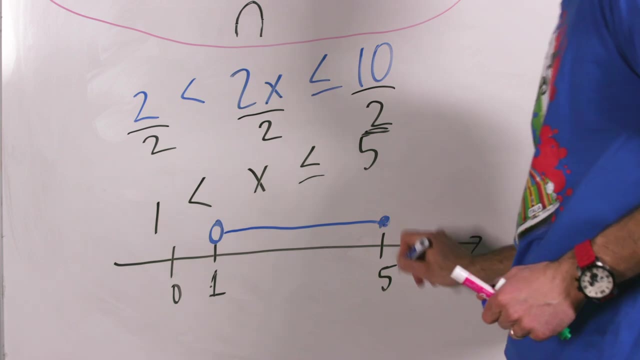 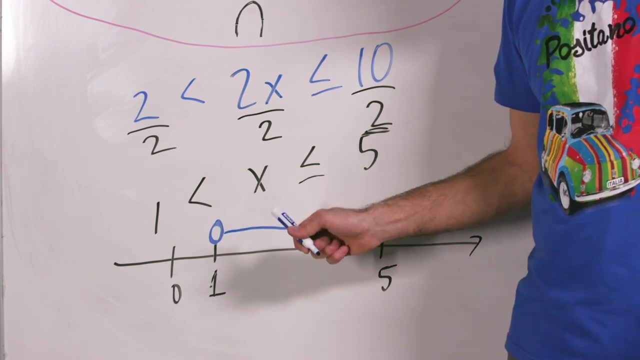 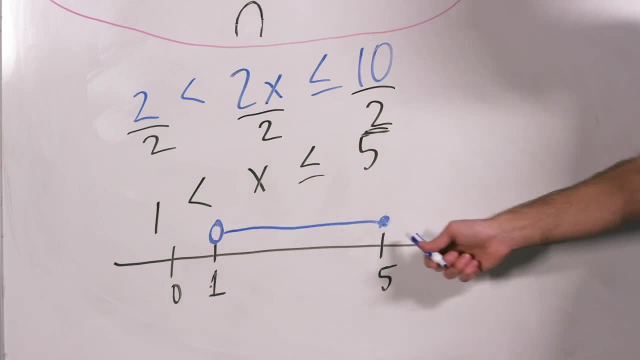 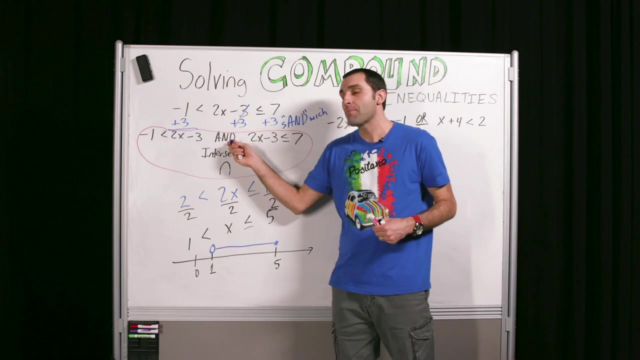 really, really close to one, but not including one. and over here, x can be 4.9, 4.99, 4.9999, 4.9999, and that's why we include five that way. okay, so one compound inequality is this concept of and the 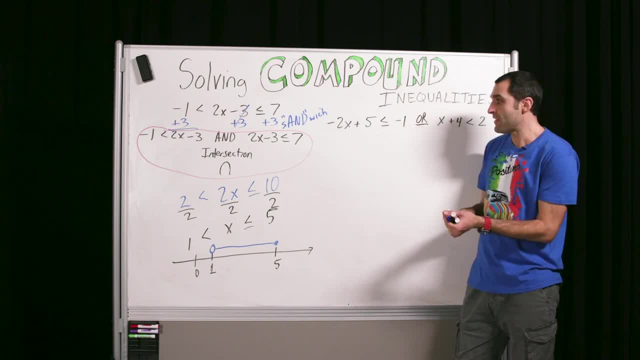 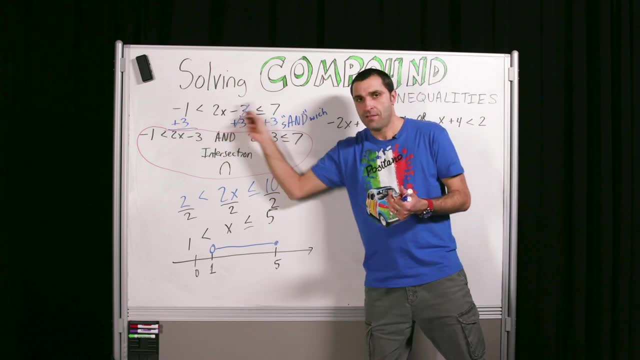 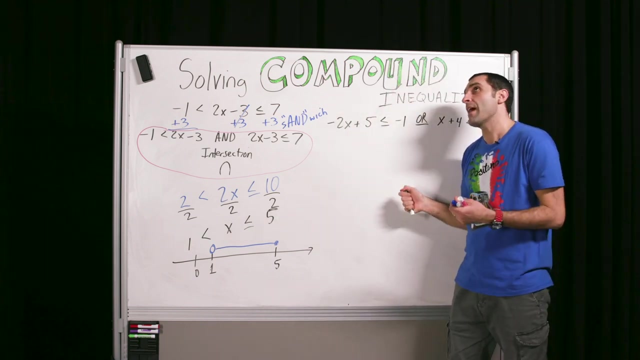 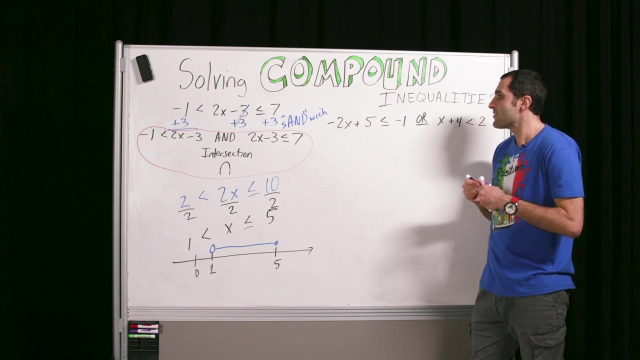 next one is the concept of or. let's put this one down. you can't do an or statement as a singular statement. it won't work, because sometimes both are true and sometimes only one is true. in fact, sometimes none are true. so in a sense we have to be ready to, uh, to like, separate them. 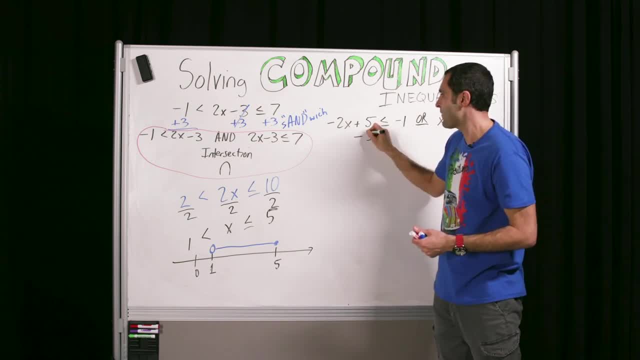 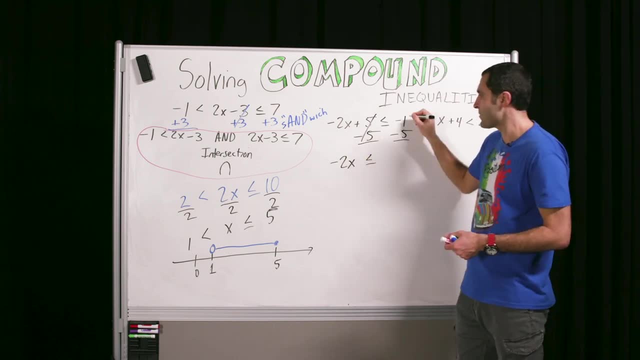 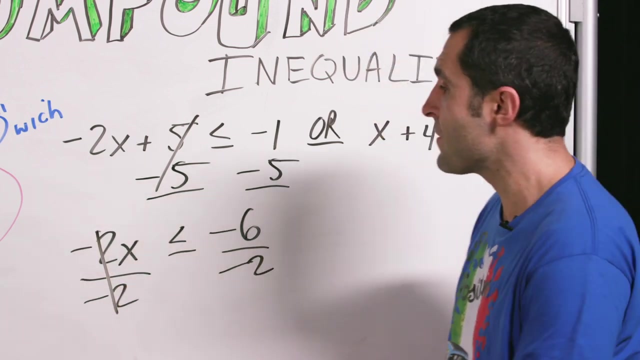 that's the idea. so let's go ahead and go minus five minus five, solving for x in the house of negative two. x less than or equal to negative. one minus five. negative six divide both sides by negative two. whenever dividing both sides of an inequality by a negative, this sign 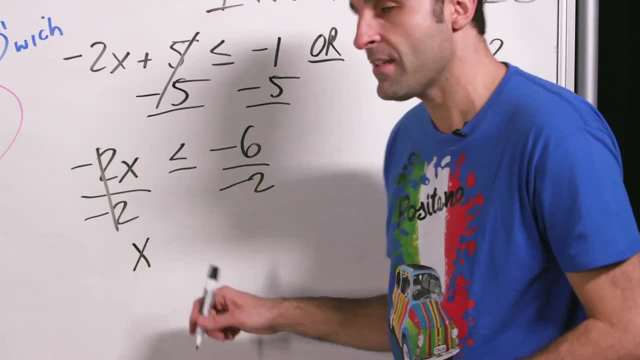 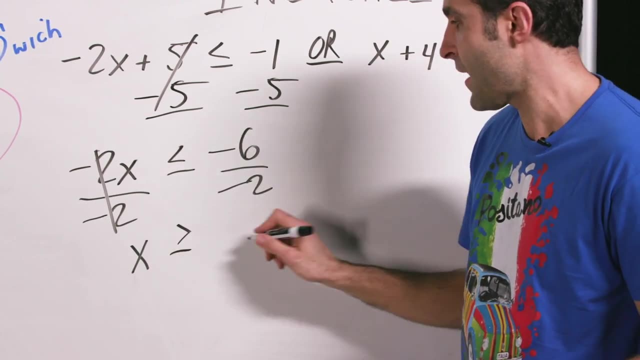 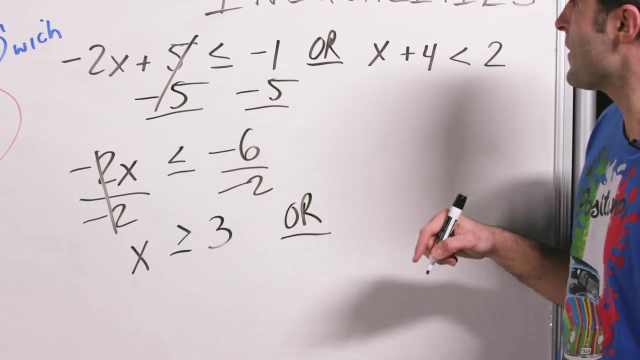 flips. there's a video on solving inequality so you can check that out and you could see why there's a. there's an intuitive proof as to why that happens. so negative six over negative two is three. so we have x greater than three, or let's go ahead and solve this subtract four on both sides. 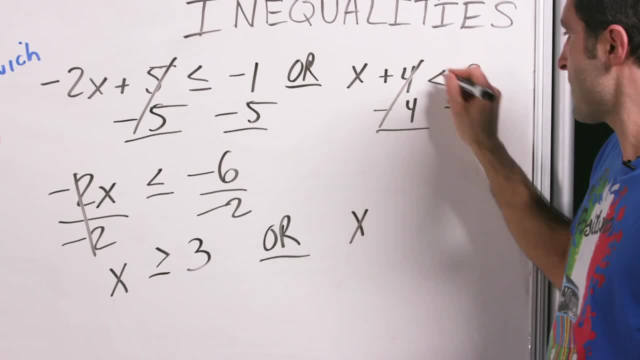 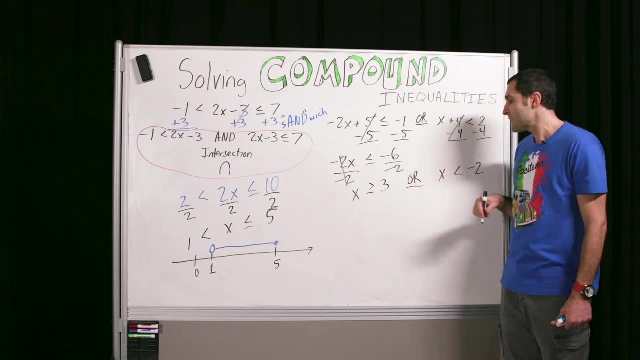 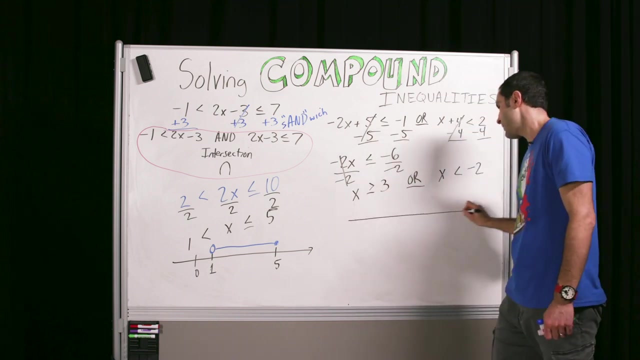 subtract four, four and we get. x is less than two minus four negative two. so you have to ask yourself: can both of these be true at the same time? so let's go ahead and solve this time. not really, not really. let's prove it on a number line, okay. 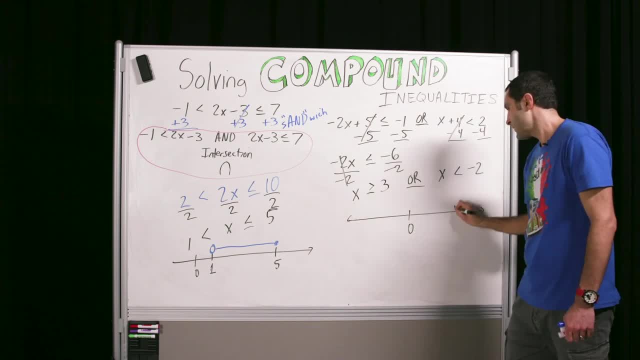 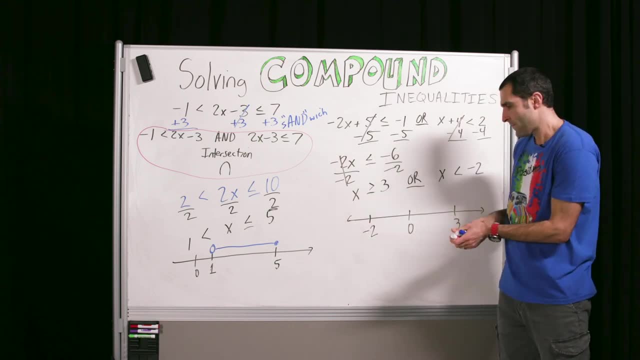 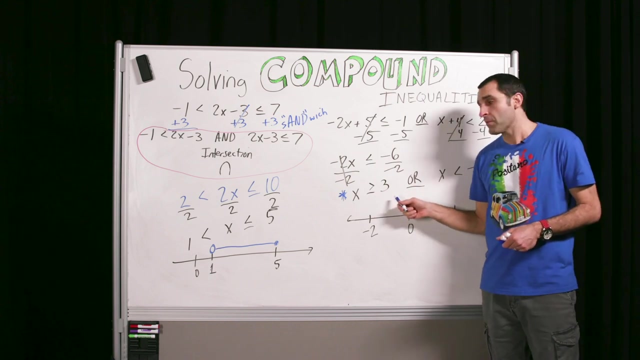 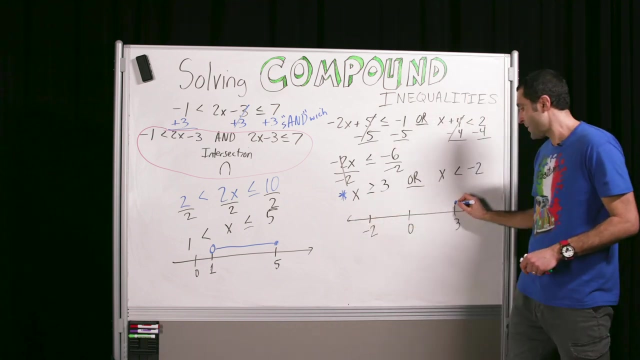 so here's zero, here's three, here's negative two. what we could do to really paint this picture nicely is that all this stuff will be the blue graph. x is three or more, x is greater than three. so we go closed circle to be greater than means bigger, bigger means to the right, and then over here say it's the pink stuff. 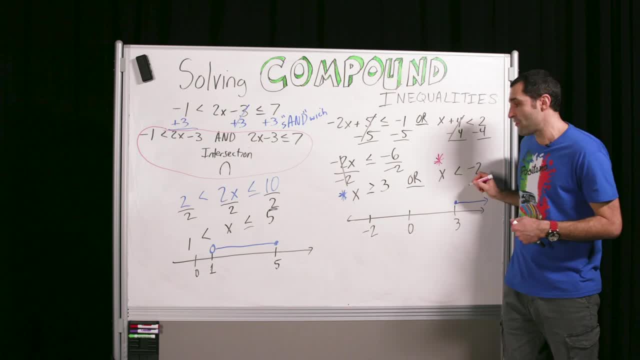 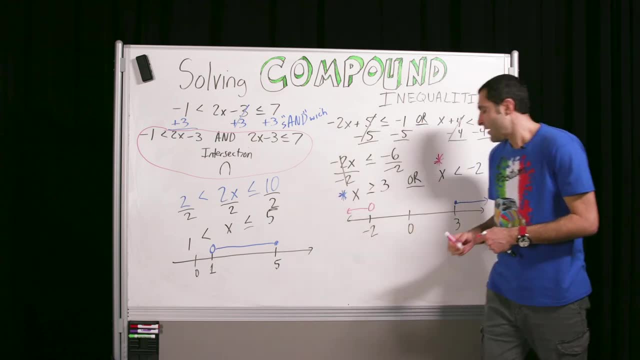 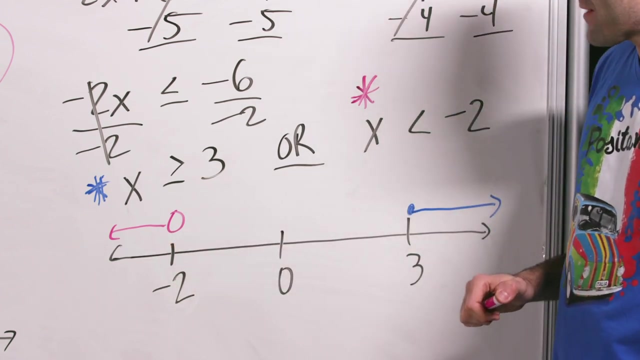 x is less than negative two, meaning not negative two, but below it. less than means small, open. and so is it possible to be blue and pink at the same time? no, it's not right. so any number that makes one of these happy will make this a true. 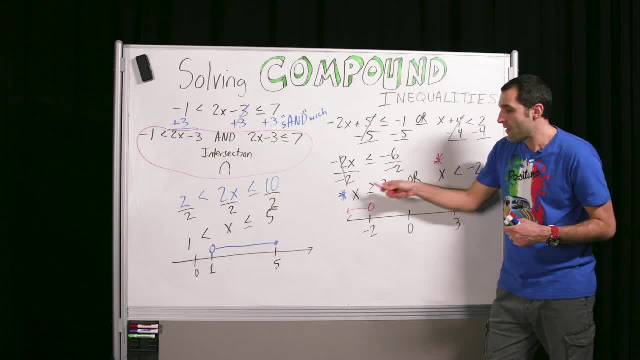 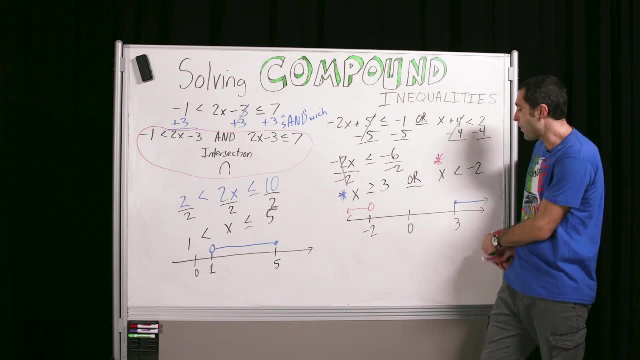 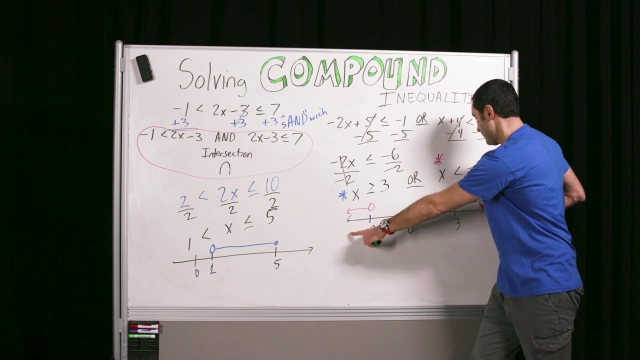 statement you think of a number like five. five is greater than or equal to three. good, so this is a true statement. x can be five, x is allowed to be five or negative five. x is allowed to be negative five. it doesn't make this happy because negative five is not blue, but it does make the pink happy because 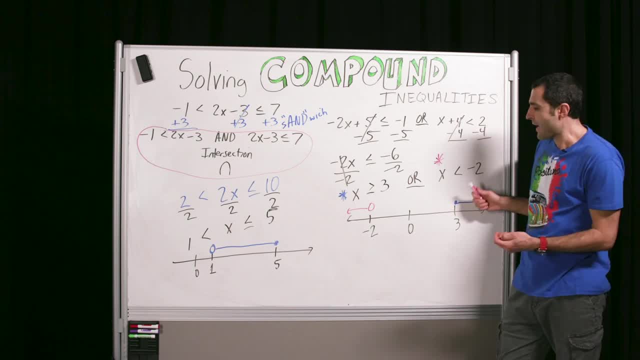 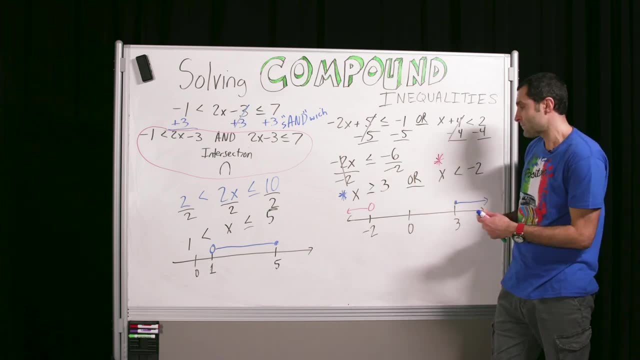 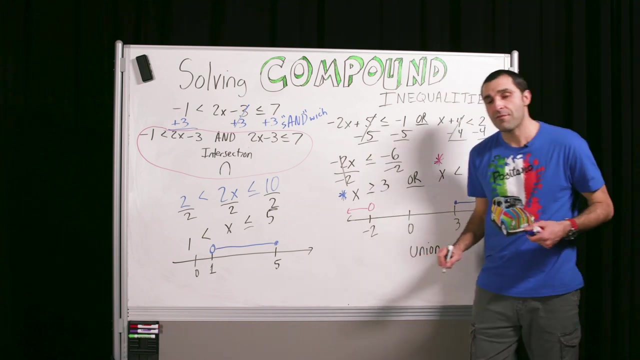 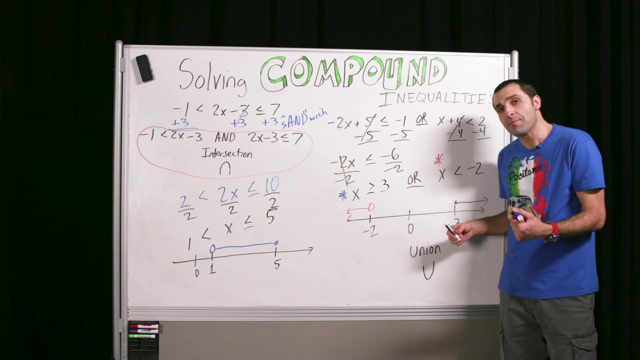 negative five is less than two. all right, so think of it that way. one needs to be true. both don't have to be so. the code word for pink is blue and the code word for pink is blue, and the code word for or is called union and union the fancy symbol for union. is you okay? in which both don't need to be true, only one needs. 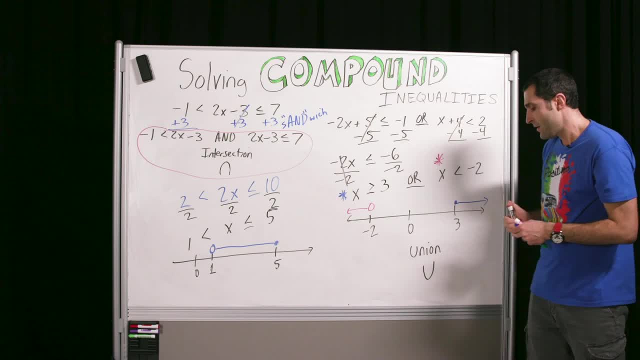 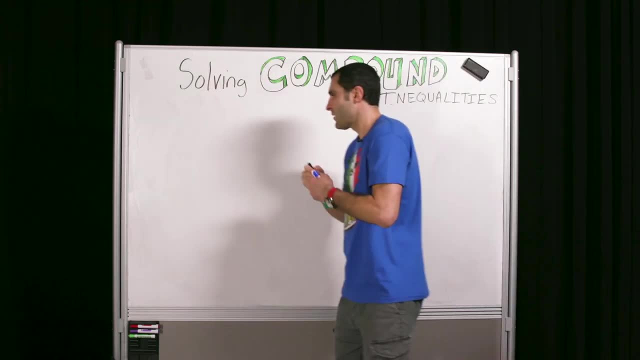 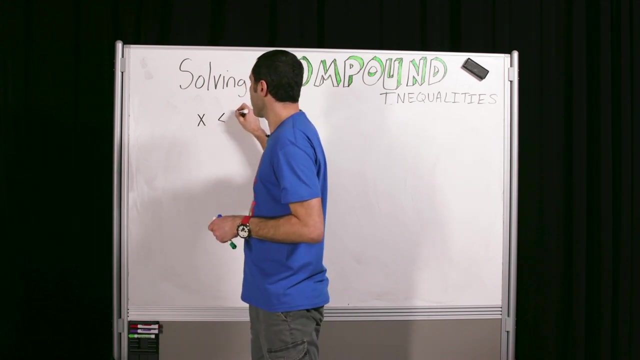 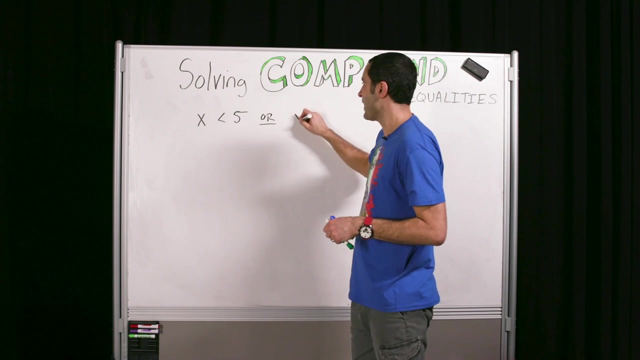 to be true, for it to be an overall true statement. okay, now i'm going to do some sort of uh exceptions with the or and the ant. suppose i had an option, myание, than makes one happy, where x is less than five, or, picking up on the or x is greater than or equal to three. 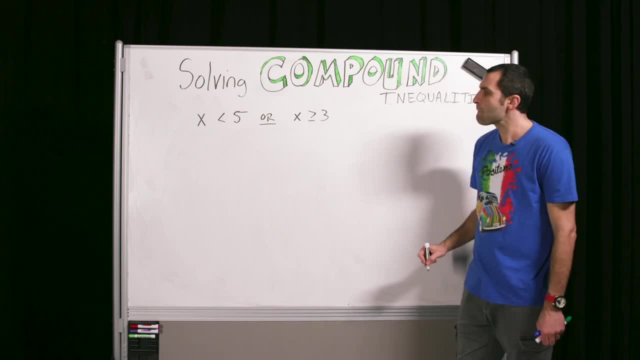 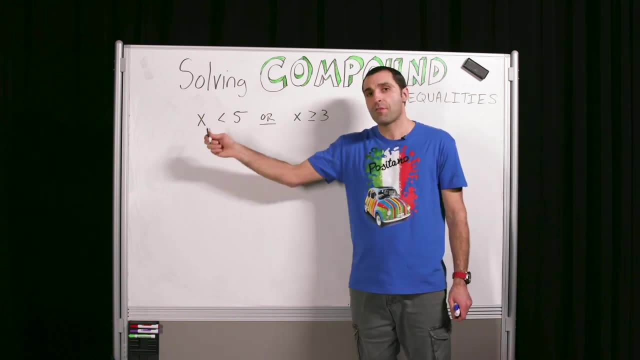 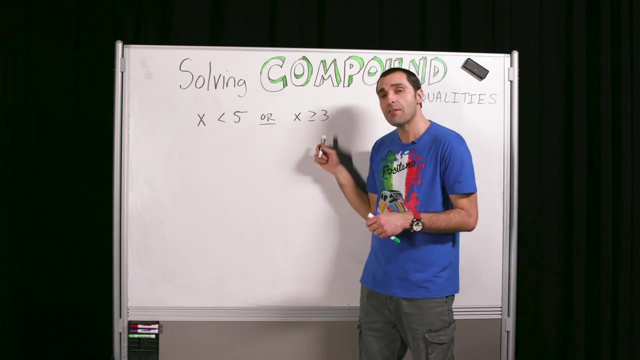 let's say: all right, we have to think what numbers make this or this or both true, because that's what or basically means. or means, if one of them is happy, other is happy, or both is happy, both are happy, then you could say the overall statement is true. 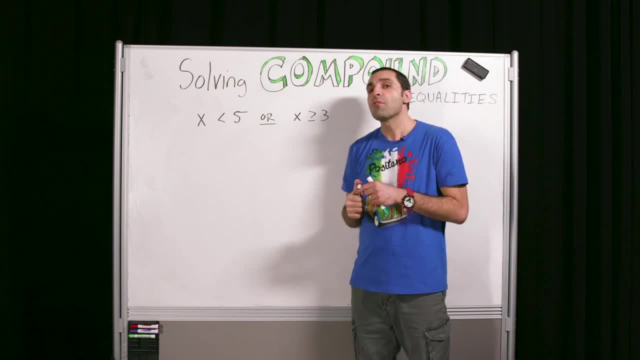 right. Kind of like a good example would be. suppose you went out Saturday night and you did not go out Sunday night, right? And I asked you on Monday: hey, did you go out on Saturday or Sunday? Your answer would be yes, because you went out on Saturday, but you didn't go out on Sunday. 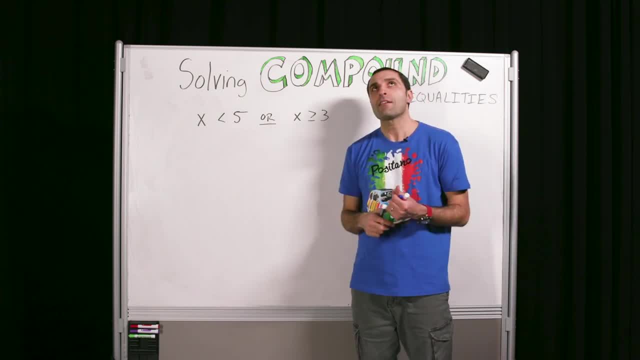 But because I asked you or you said yes, since I went out on Saturday. the answer is yes, I did go out on Saturday or Sunday. okay, But if I had asked you, hey, did you go out on Saturday and Sunday? Your answer would be no, because both would need to be true. You didn't go out on Sunday. 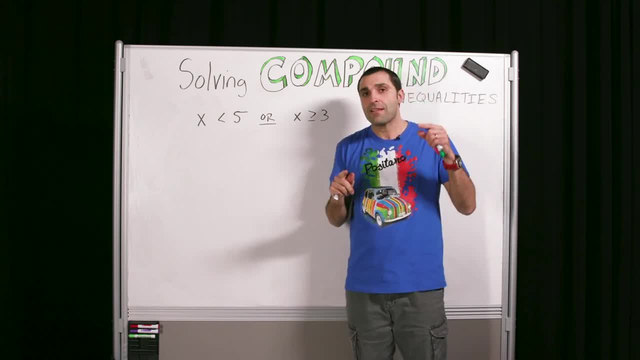 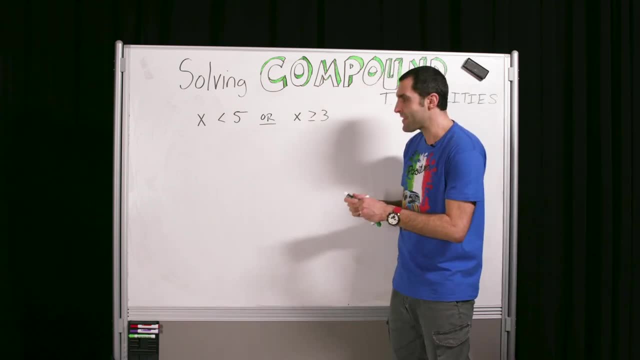 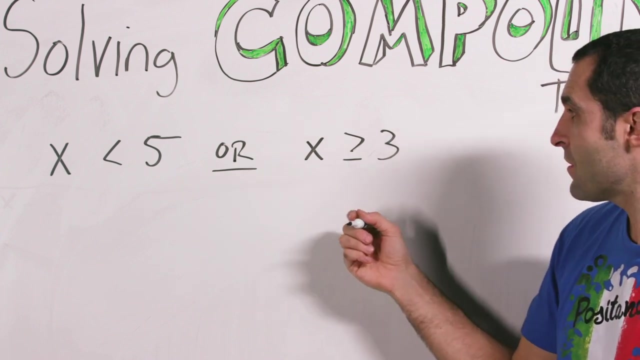 you did go out on Saturday. So since both weren't true, the answer for and is no. In other words, it's harder to do, and you know, because both need to be true. Let's see about this: or Saturday or Sunday, What numbers are less than five or greater than or equal to three? 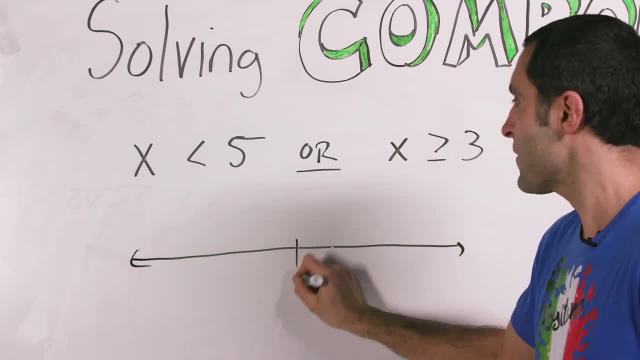 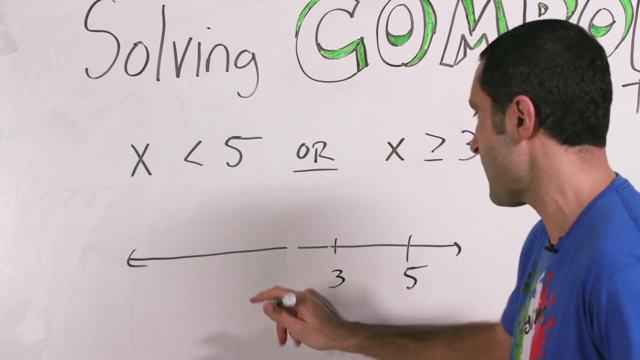 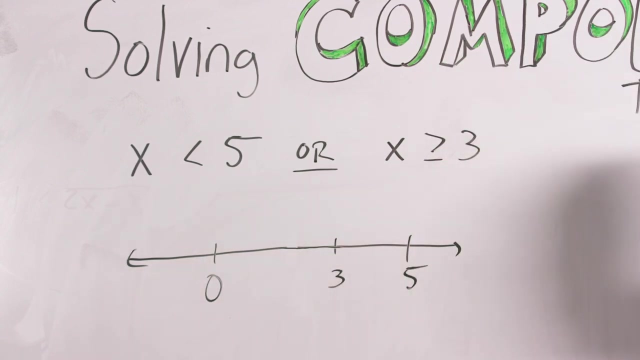 Let's check it out. Here's zero, here's five, here's three. I'm gonna move zero a little over a little space. That's good. Okay, less than five. we'll make them blue, All numbers. less than five. 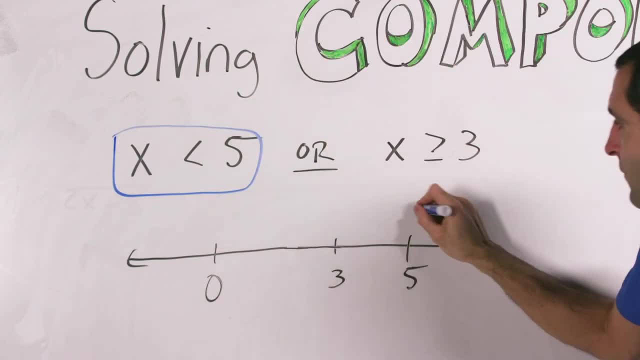 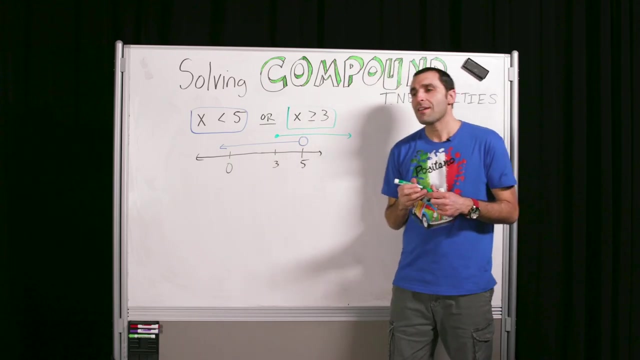 Put that in a little box: Five open circle. less than means left, All right. And then three greater than or equal to three is in green, So we can go closed. Greater than means right, Cool. What numbers are less than five or greater than or equal to three. In other words, asks what numbers. 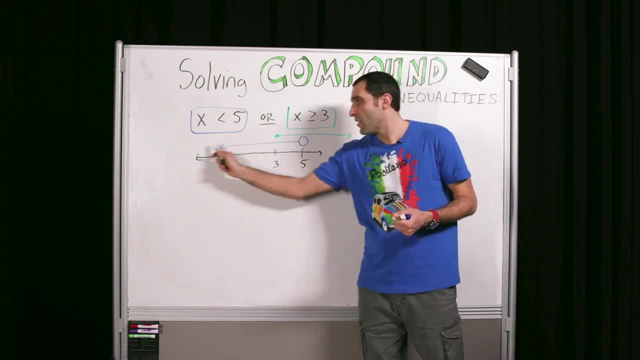 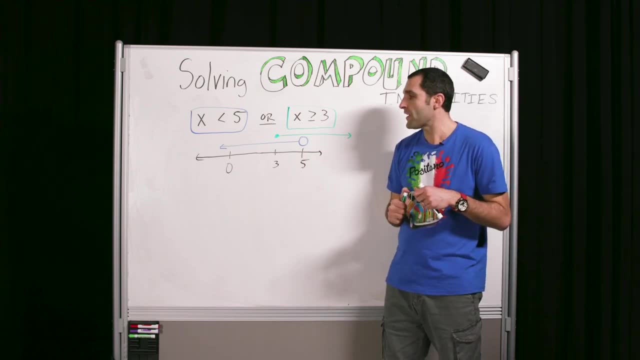 are less than five or greater than or equal to three, Are blue or green or both. Can you think of a number that's blue or green or both? I could think of a lot of numbers that are blue or green or both. you know, like zero. 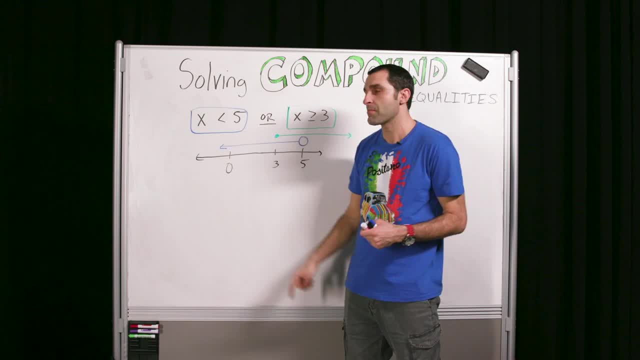 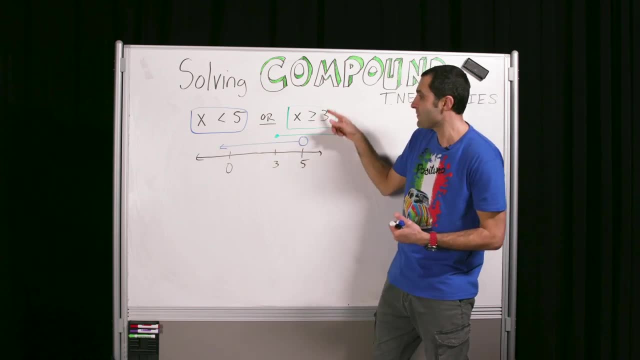 Zero is blue. Zero is covered by the blue line, So zero is blue. That means zero makes blue happy. Is zero less than five? Yes. So it doesn't matter that zero doesn't make this happy, It doesn't matter that it's green, Zero is not greater than or equal to three, but zero works. 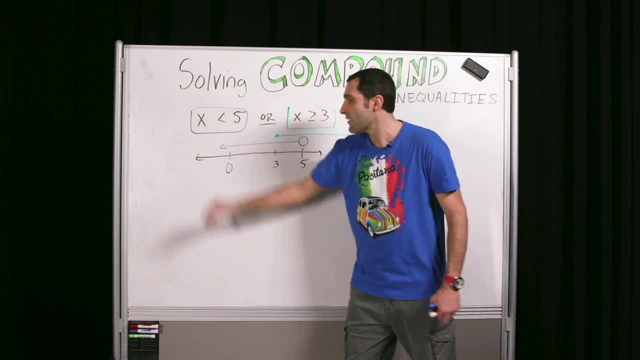 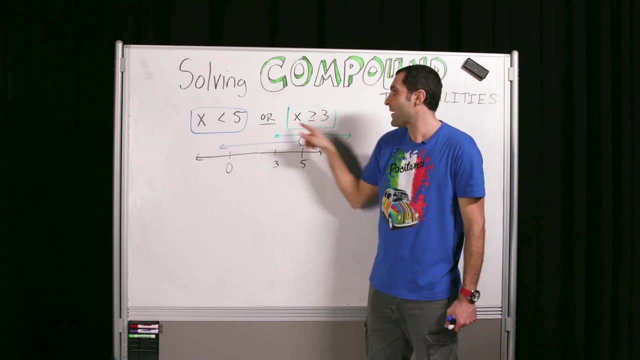 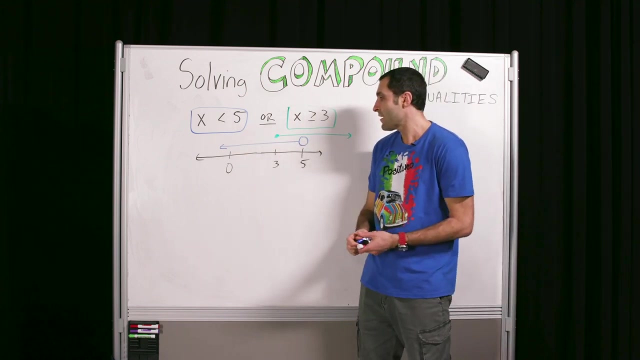 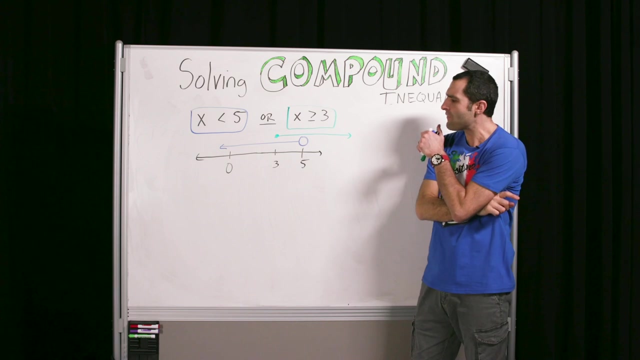 Zero is a solution to this compound inequality. What about four? Four makes this happy. Four is blue. Four makes this happy. Four is greater than or equal to three. So, since it makes both happy, four is a solution. What about ten? Ten is green. Ten doesn't make this happy, but ten makes this happy. So I tried every single number I can think of. 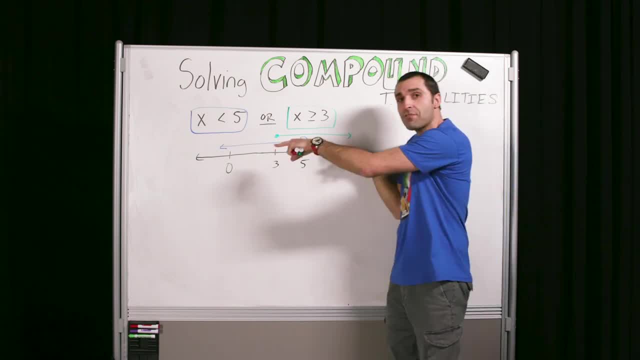 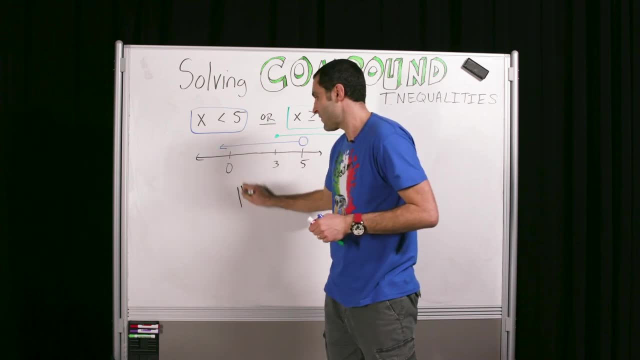 Is blue or green or both, Every single number is actually covered. So the answer to this compound inequality is all real numbers. Here's the fancy symbol for all real numbers, The capital R with two lines. You could try drawing it. It's fun. 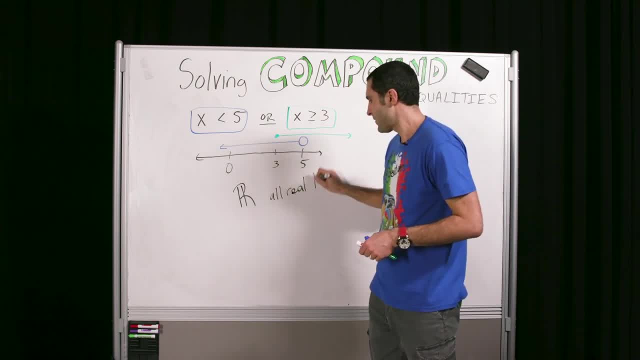 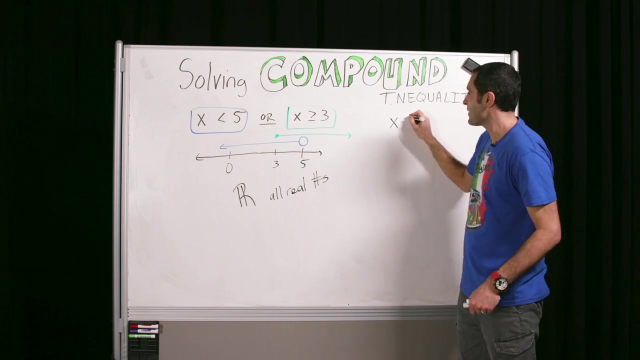 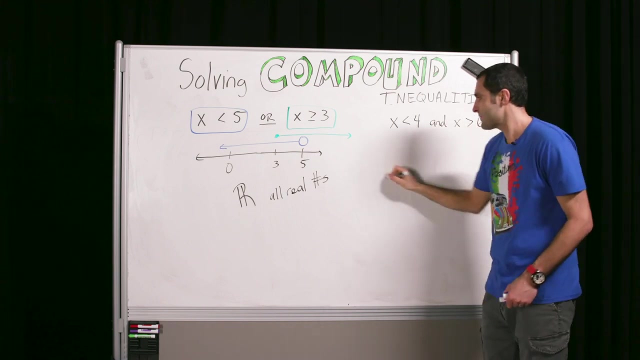 All real numbers, Meaning any number will make one or the other, or both, happy. Okay, Let's try a different one, though What if I said X is, let's go with, less than four, and X is greater than six? All right, So here's zero, Here's four, Here's six. 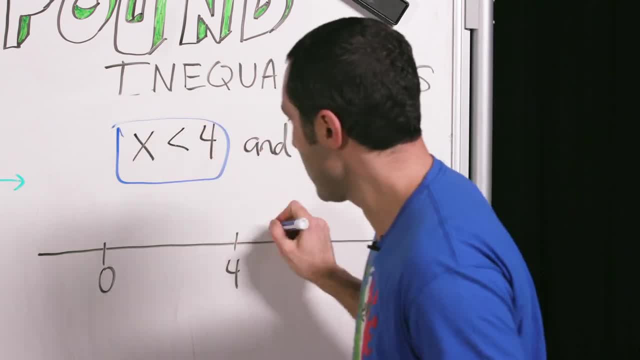 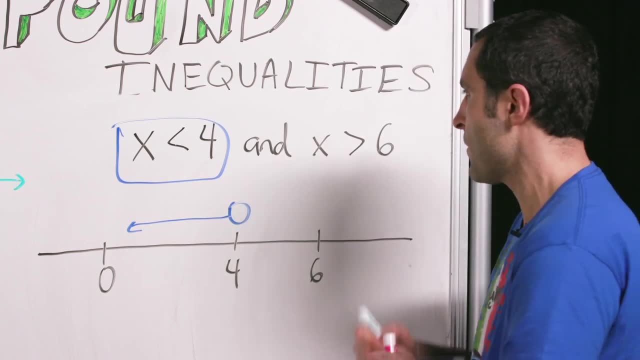 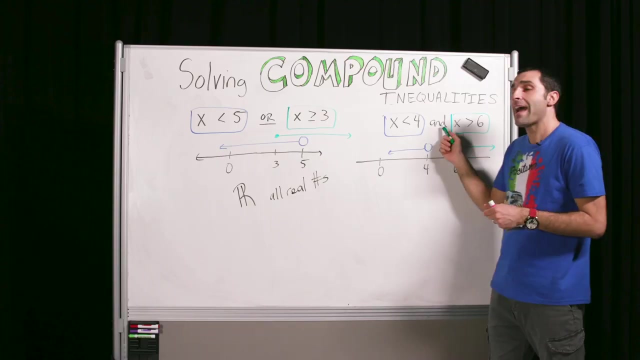 Let's go with the blue again. This is blue. Open circle on four. Less than means small, All right. And then this: this one was green open circle on six to the right. There it is So. and asks: both need to be true, All right. 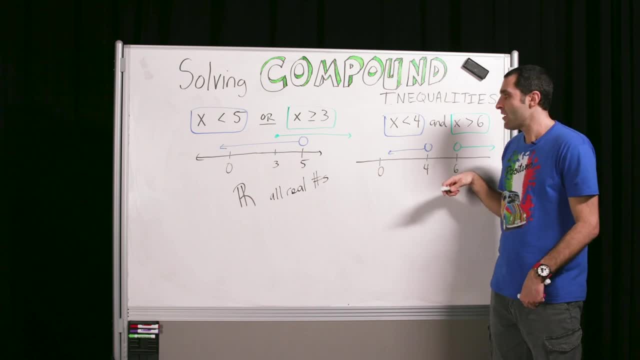 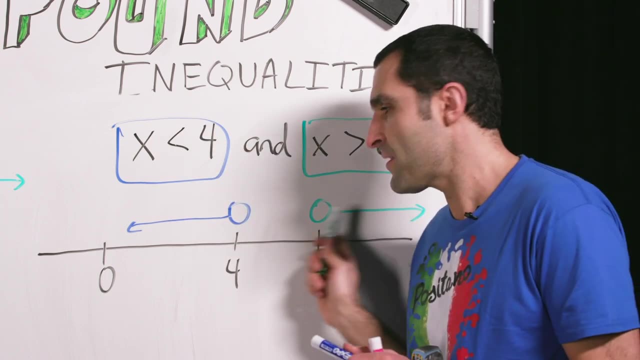 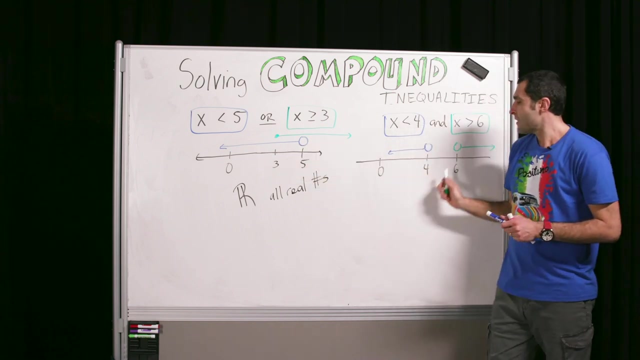 So what numbers are blue and green? What numbers are both less than four and simultaneously greater than six? Can you see numbers here that are blue and green at the same time? I saw them here. Okay, Let's try a different one. 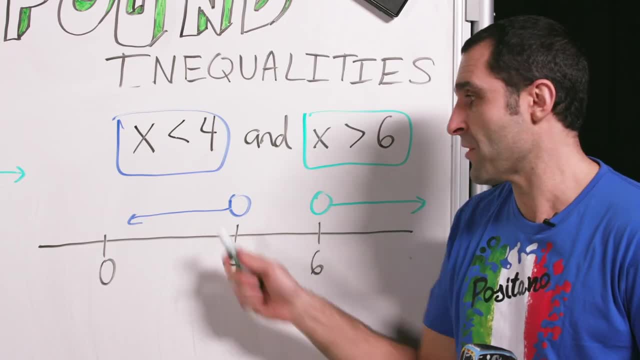 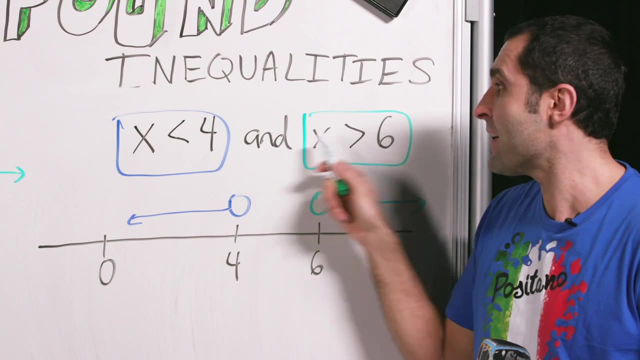 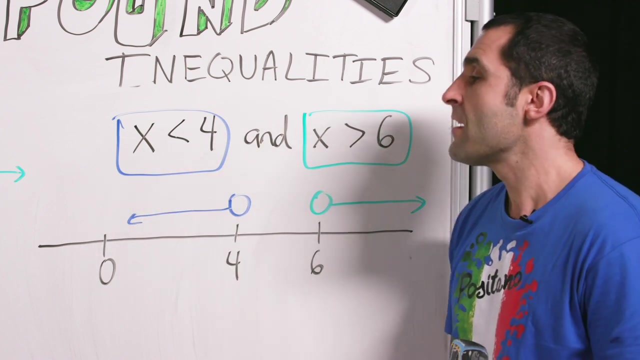 seeing them here. It turns out there are no numbers that are blue and green at the same time. There are no numbers that make this happy here and this happy simultaneously And since and needs both to be true, there is no number that makes both true. Try as we may, You know we could. 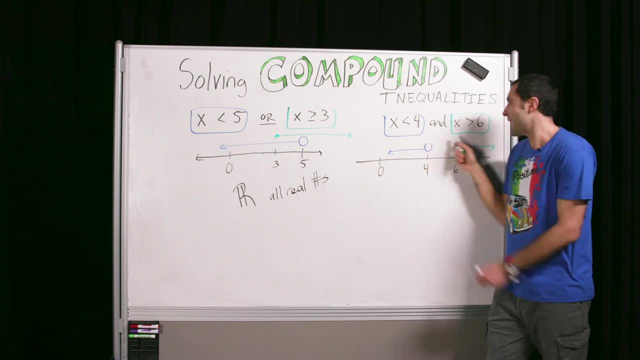 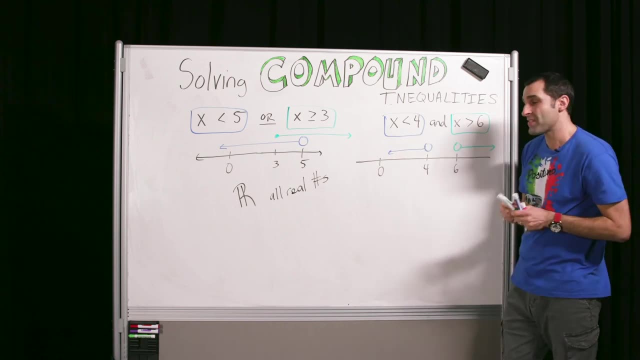 say three, but three doesn't make this happy. We could say ten, Ten makes this happy, Ten's greater than six, Ten's not greater than four, So on, this is like the opposite side. So no solution, No solution, All right. So now I'm going to ask you to get your bodies involved in this learning All. 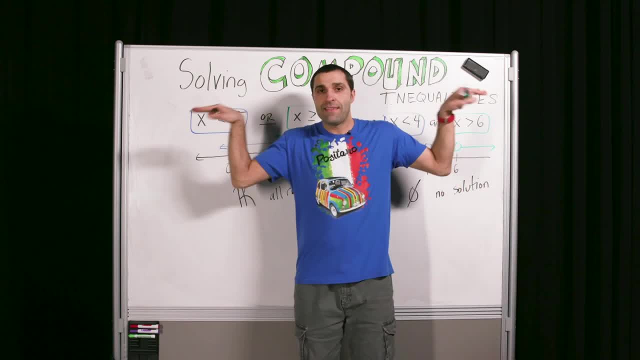 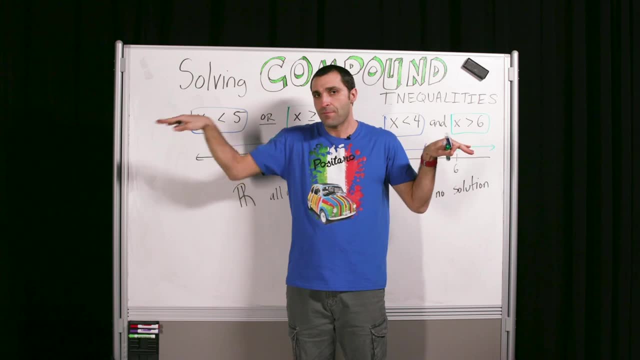 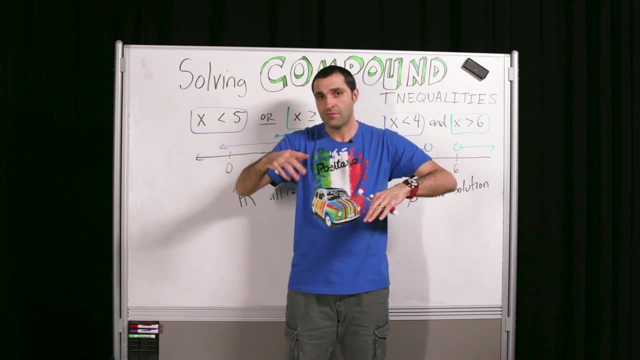 right, So let's give it a whirl. If or goes like this, that's cool. Okay. If or goes like this, that's cool, Because numbers are either here smaller than something or greater than something, and not both. If and goes like this, that's cool. If and goes like this: 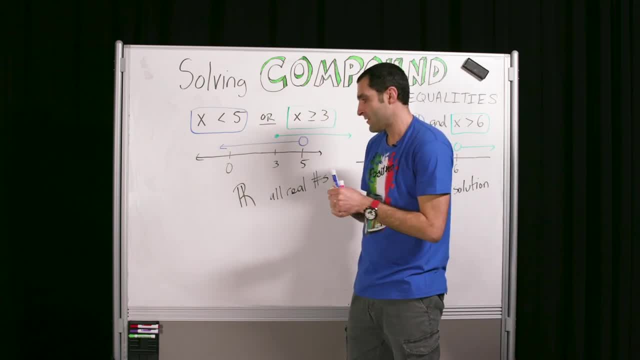 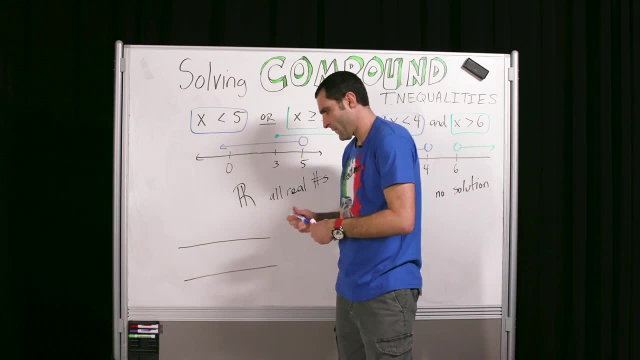 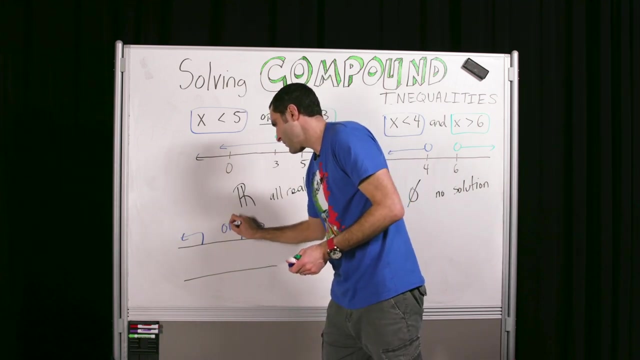 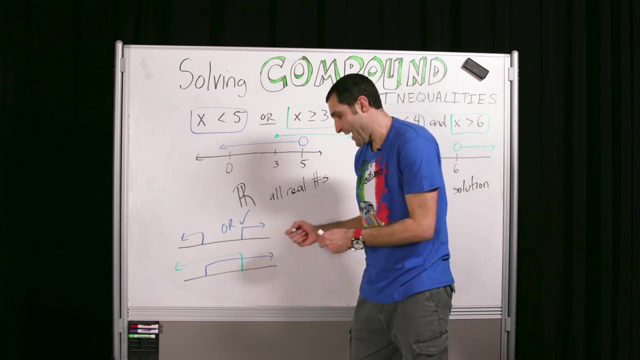 we're thinking: what the overlap is, All right, So let's actually get those. So here's when. or going like this, Let's do it, That's fine. Or going like this, Or going like this, That's fine. This is a fine answer for or So we go here. And then we go here. And if this was an and problem. 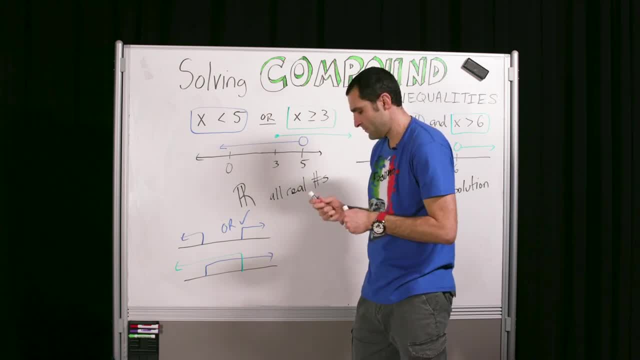 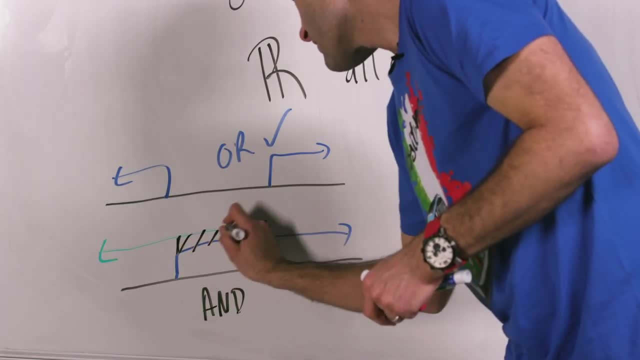 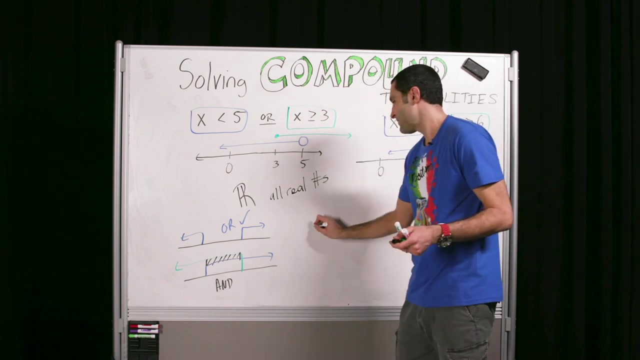 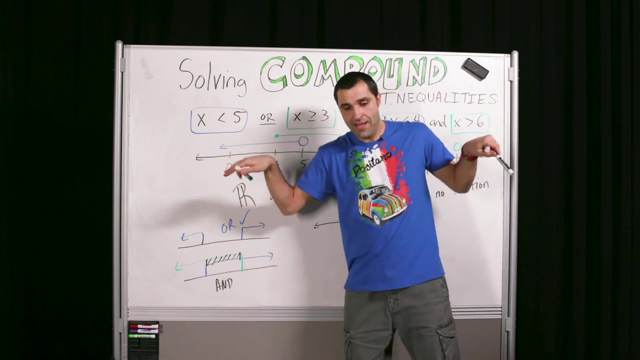 that's cool Because. and asks about overlap, And so the overlapping section would be this: So that would be the final answer. You could shave that part. Some people erase it, so that's cool. but this one here: what happens if you have and like that try. 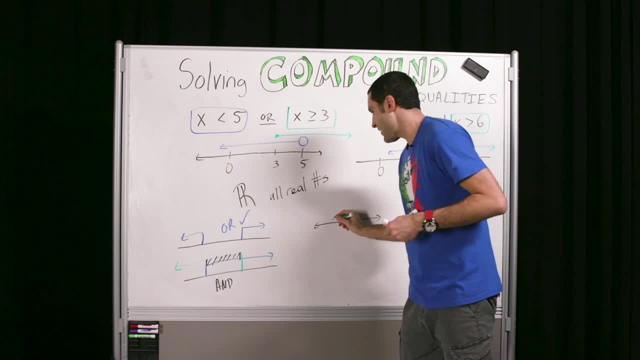 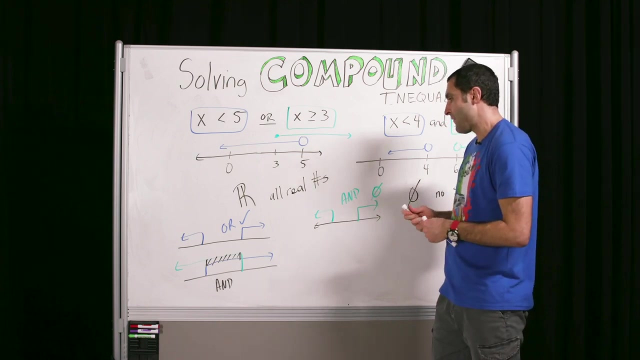 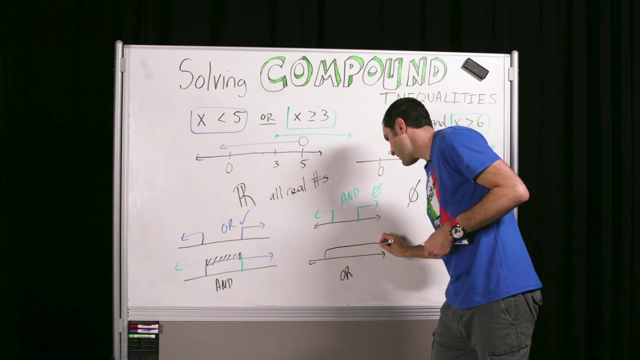 that, and is it possible to have overlap here with this? and so this is a, never an, and problem when they diverge like this. this is no solution. and then, if you have an or that's converging, yeah, or going like this as well as this, what numbers? 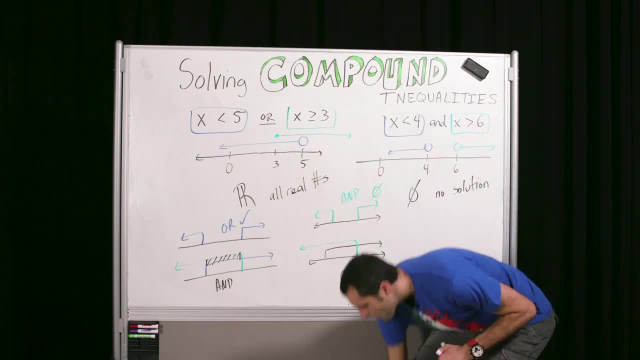 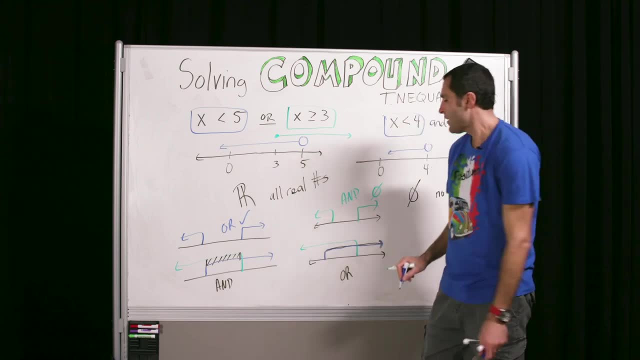 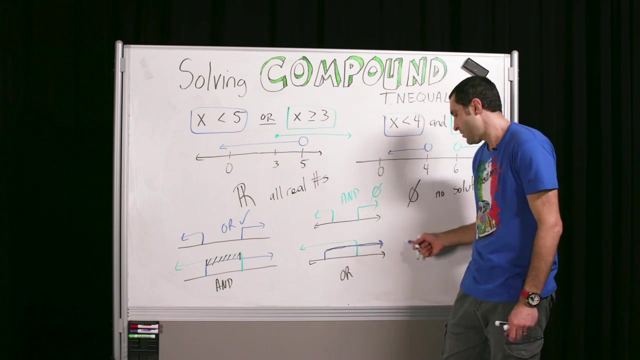 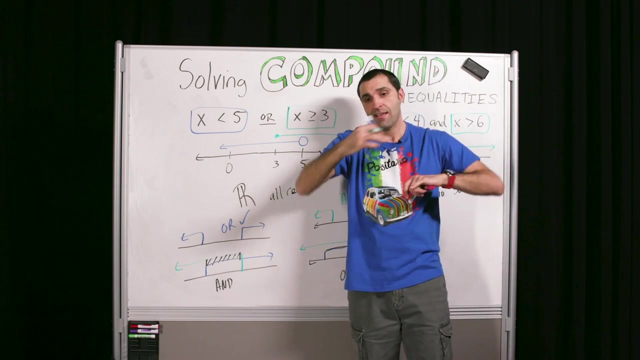 are covered by. let's go pick a different color here. what numbers are covered by black or green? we'll say blue or green. what numbers are blue or green or both? all numbers are blue or green or both. So in this case, when you have or going like this: that: 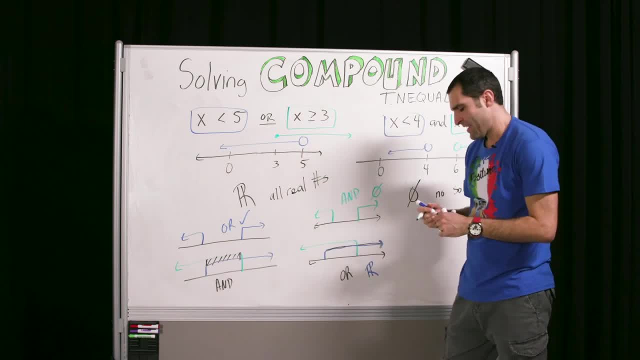 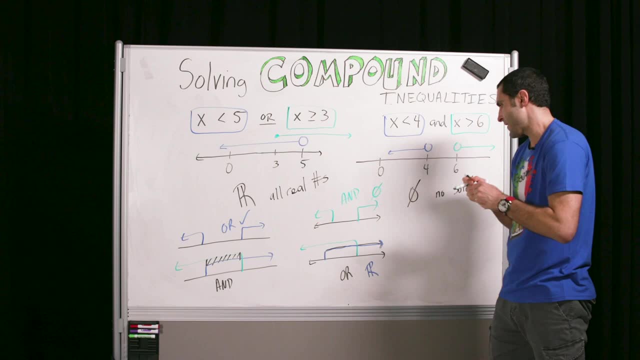 would be all reals. That's essentially all the major ones you know- And you could think of other ones- that sometimes they go in the same direction. You can handle those right now. Give them all to you So you have them all good to go Give. 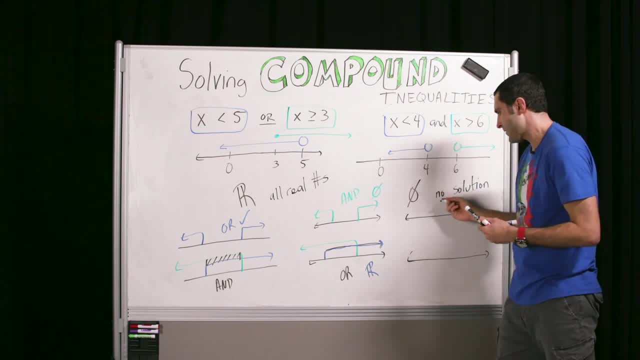 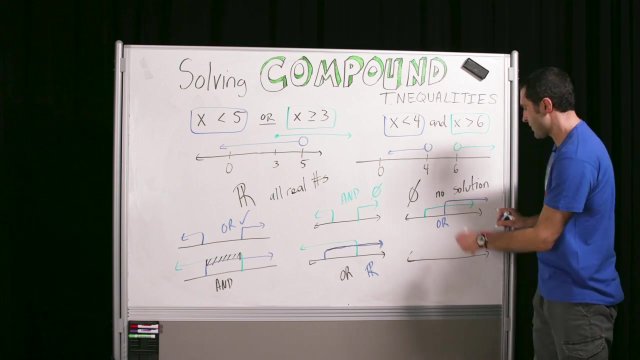 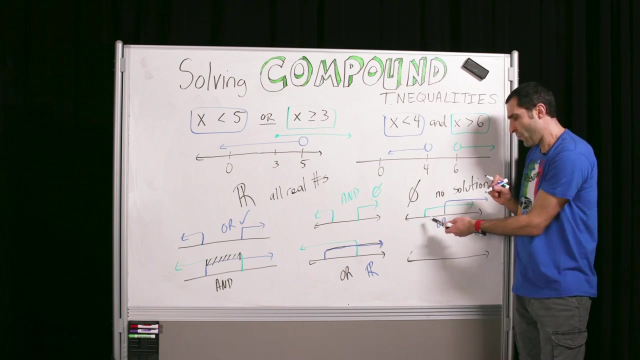 them all to you, So we have like here and here. So if this was basically or, you could just kind of leave it. you know, If that's or that's fine, Technically it's, you could start from here. Only one needs to be true, or both. So or it's. 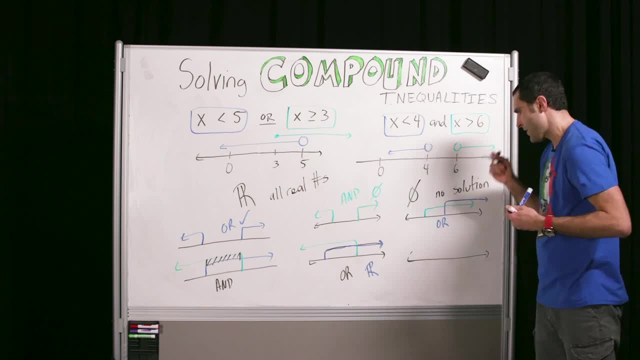 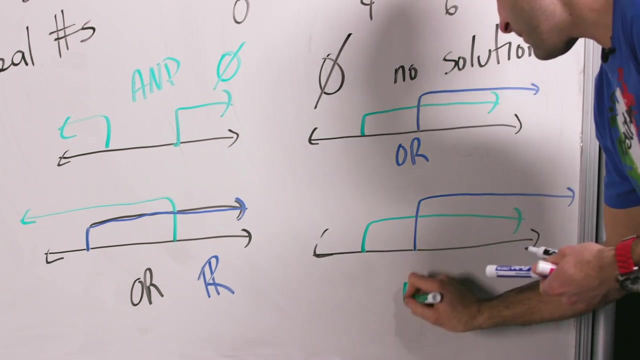 fine to just leave that. You know there's no, there's no harm in that. Okay, But with and right we have here boom and requires overlap. So if this was an and problem, we would have to explicitly shade. 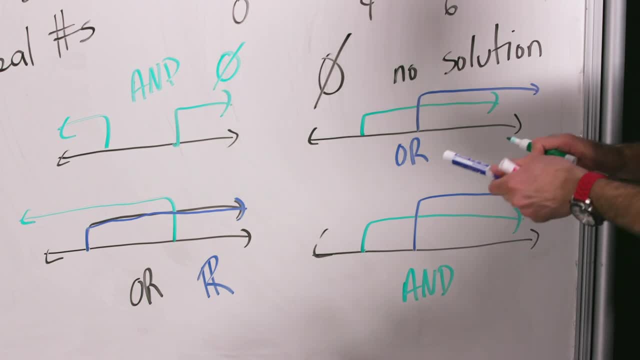 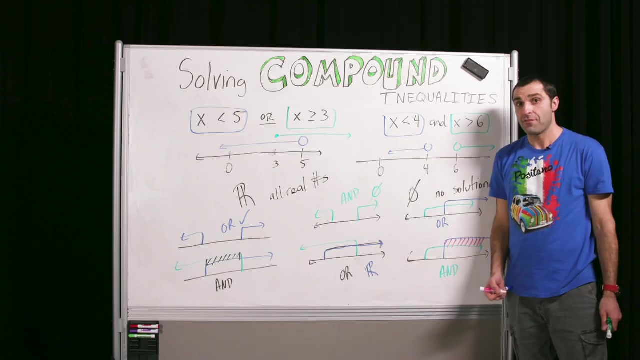 Let's do something like: I'll pick the pink again. I'm having a lot of fun with these caps, Mix and match and pink and green here. So we have to explicitly shade the overlap for: and So that's really every, every, every scenario, okay. 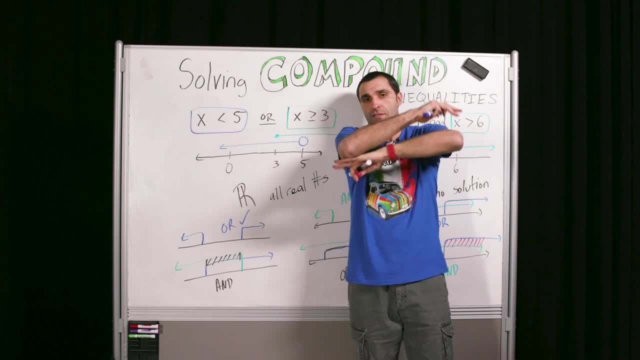 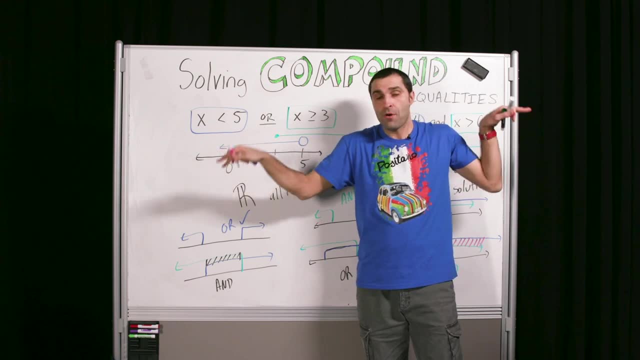 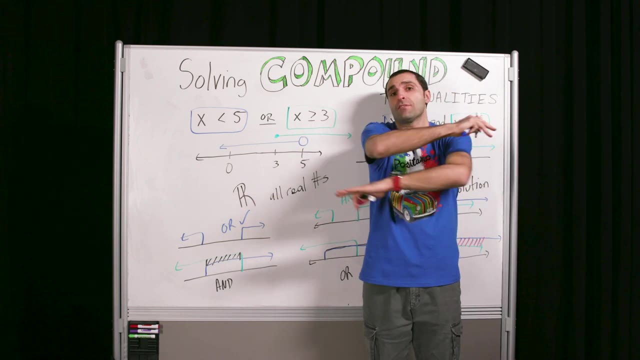 Or going like that cool. And going like that cool, overlap, shade them or erase the sides. And going like that basically not cool, impossible for both to be covered like this, So no solution. Or going like that kind of weird because all numbers are covered here. 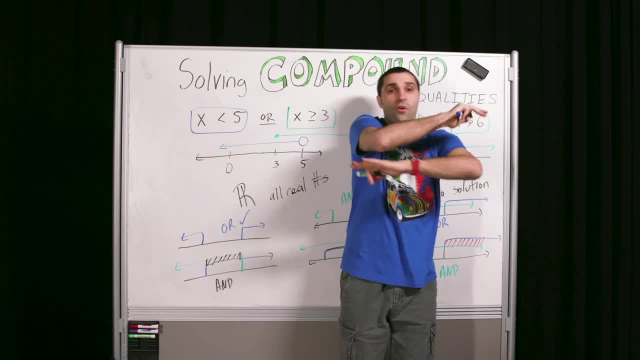 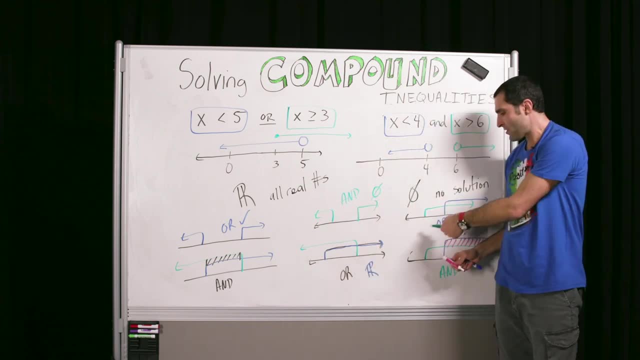 All numbers are covered by this Or by this, Or by both. So in that case, or converging is all reals, And then when they go in the same direction or is fine, You know- overlap, or one, And though it requires a bit of shading, okay. 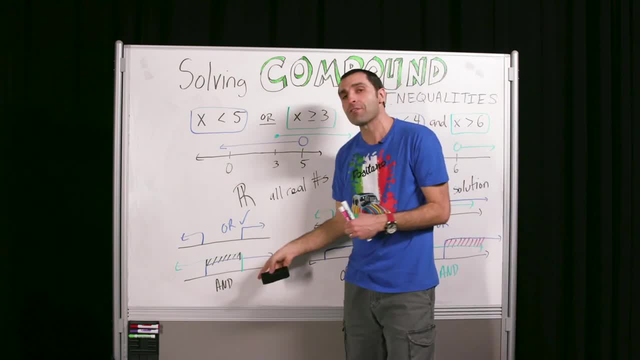 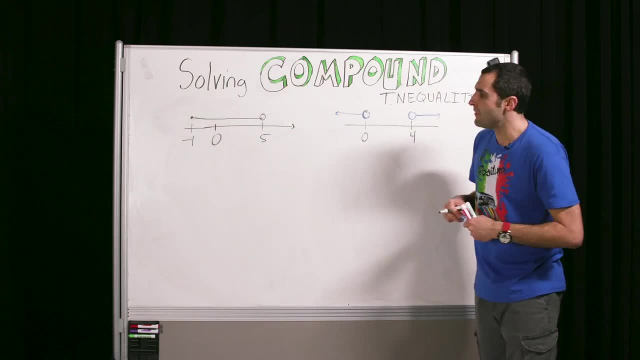 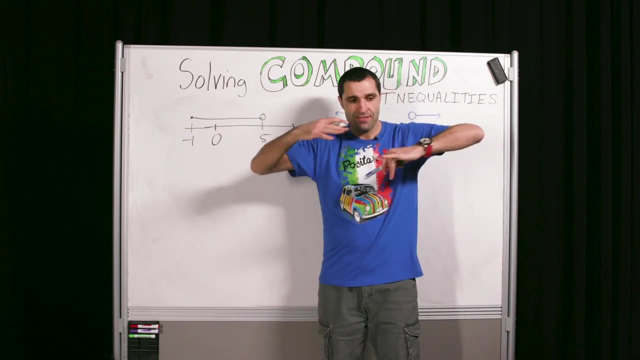 The last thing we'll do with regards to this is, if I gave you the graph, you come up with the compound statement: right, All right, Or, or, and, Or, or, and. Traditionally, This looks like an and. because it's like an and overlap. 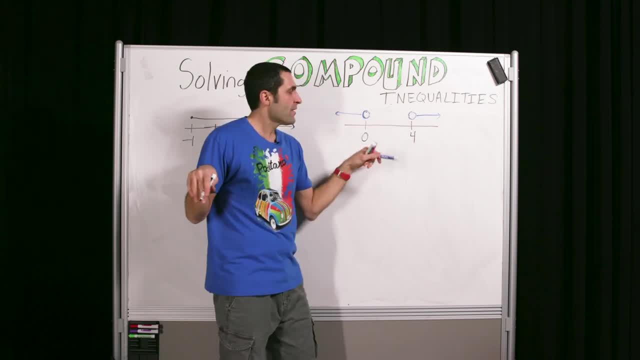 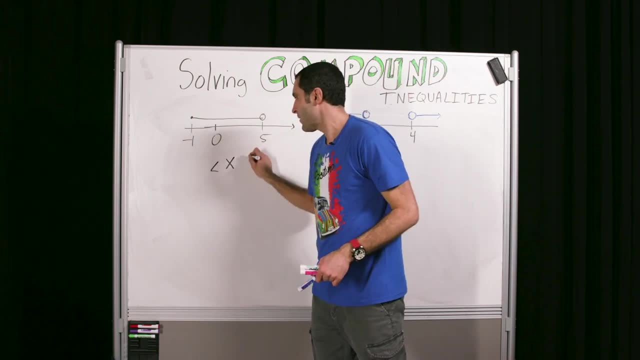 It's not looking like this, where one or the other can be true. So I'm feeling like this is an or and this is an and. Since it's an and, we can do the and which. Boom, This is pretty much the format for the and which, in which we're or, equal. 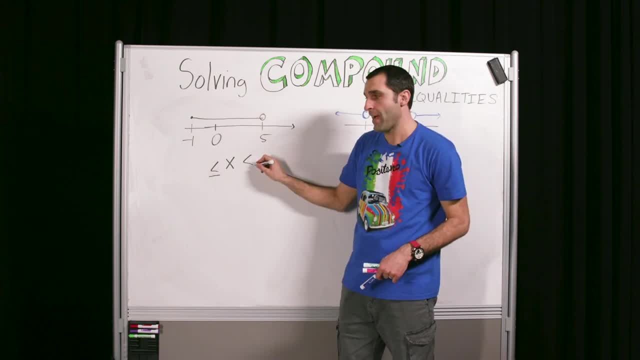 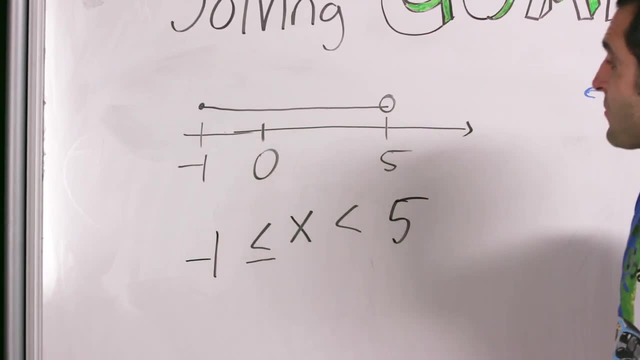 to the bottom. one and not or equal to five Go small to big in this case, Small to big. So we put negative one. here We put five And it's true, X is now greater than or equal to one, Meaning above negative one. excuse me, 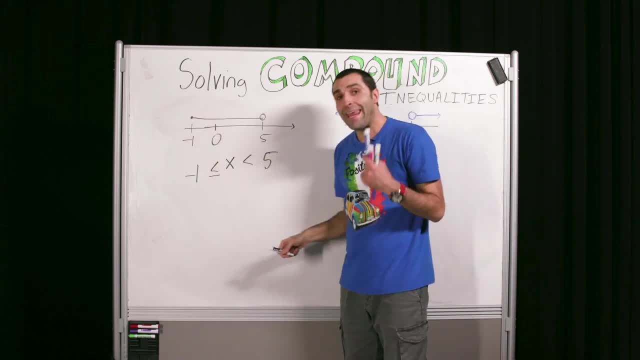 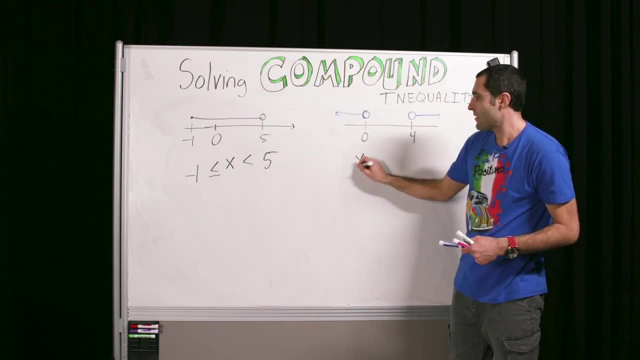 X is greater than or equal to negative one here to the right And X is less than five right, So both of these are true, Whereas over here X is what? zero, Smaller or bigger? Well, we're looks like we're going to the left, so that's small. 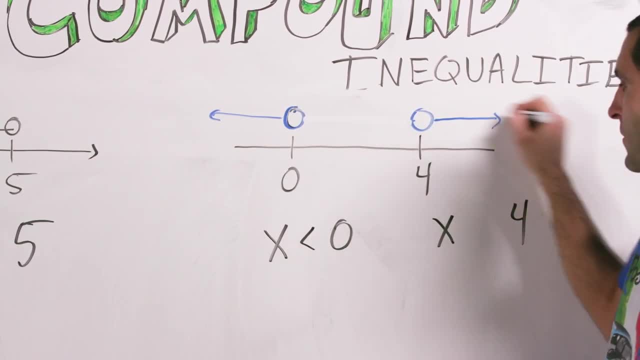 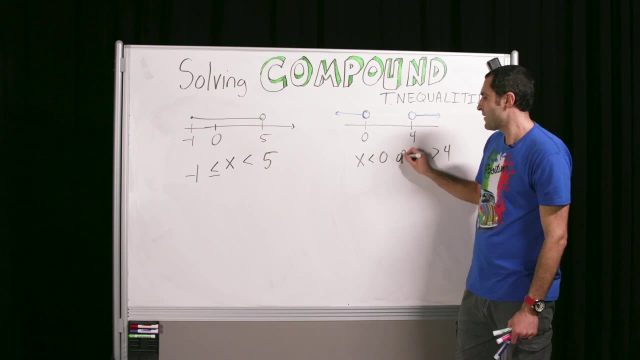 X, is what here? Smaller or bigger than four? Looks like we're going to the right, so bigger. Can both of these be true at the same time, Or There you go. This is an and statement. All right, cool.